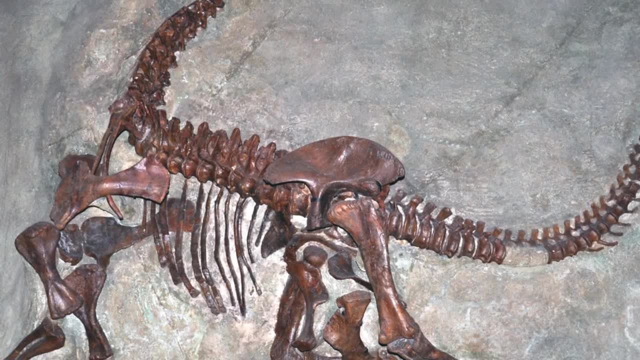 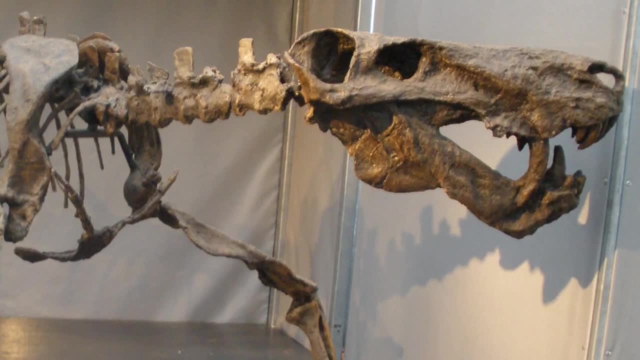 These words are not meant to be confusing. In fact, they're applied in order to better describe whatever it is that's being discussed in a more precise manner, But I remember how puzzling it was when I was younger to be confronted with these unfamiliar terms littered throughout paleontological discussions, and how 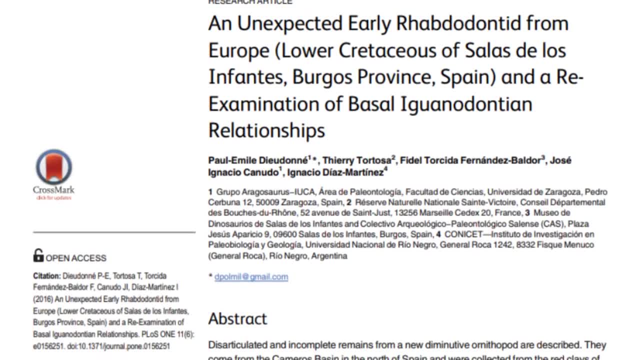 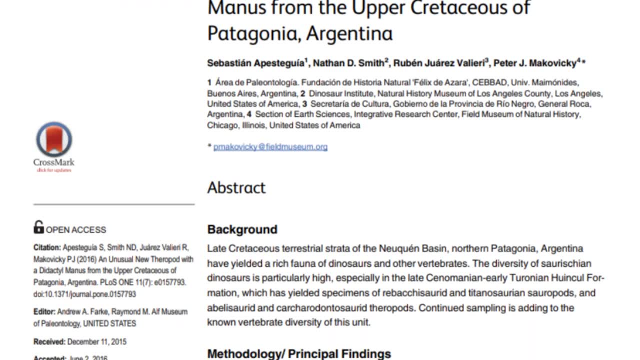 often I'd have to search up the meanings. I found that the best way to become better at understanding what everything meant was to just keep reading scientific papers and googling anything I didn't recognise. I would still recommend doing this, as it's a 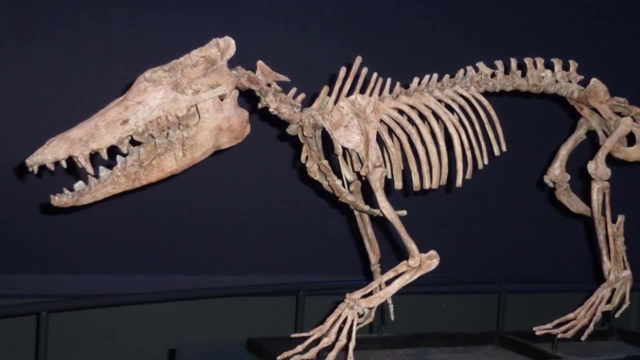 very effective way to study. but to help others who might be wanting to learn about the science like I did, I thought I would make this video as an introductory video to help you learn more about the science of paleontology. Thanks for watching and I'll see you in the next video. 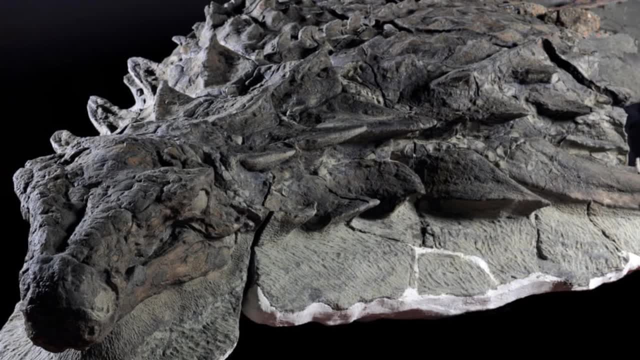 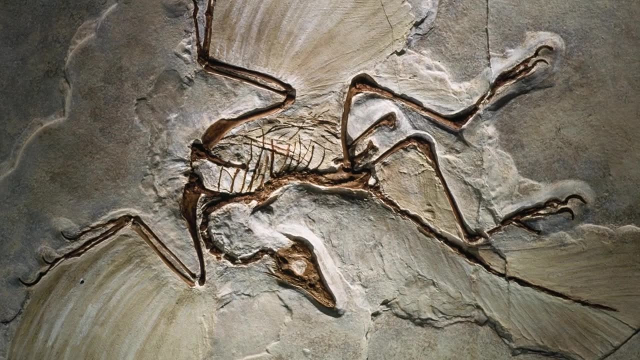 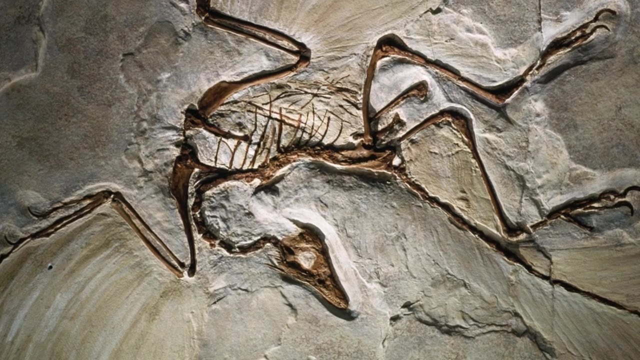 So let's get right to it. First of all, there are the names of the various areas of study within paleontology itself. I remember these terms being particularly confusing to me when I first came across them, since they seem very complicated But in reality, 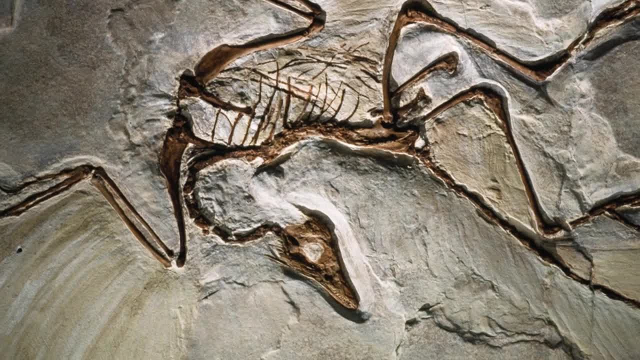 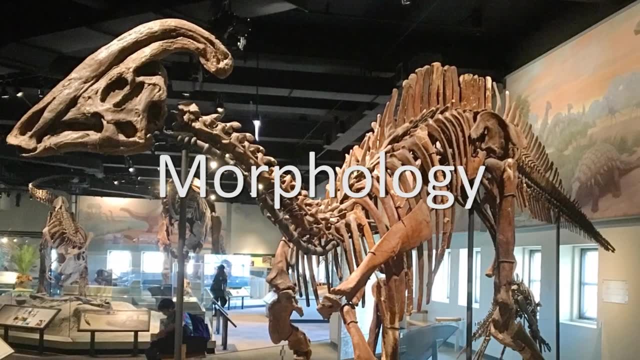 they're just describing which part of the science is being applied in a certain situation. For example, morphology is just the name for the studying of the physical shape and structure of an organism In paleontology. this is likely to apply to fossilised bones or 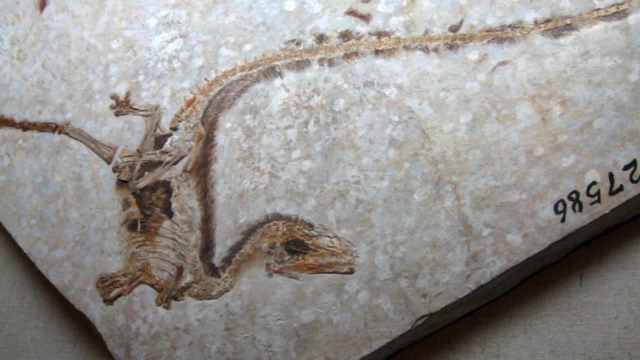 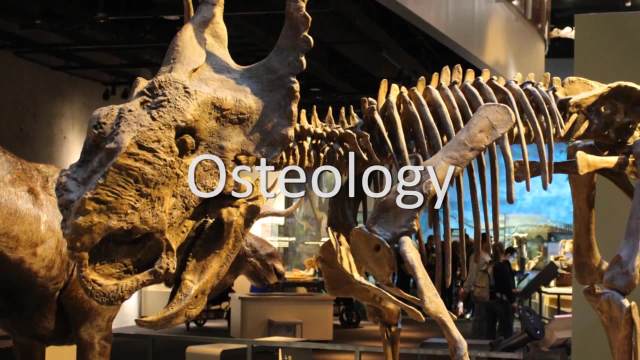 soft tissue, which can be morphologically analysed to describe their exact forms. Osteology is sort of similar to this, as it's the study of how the skeleton works and is structured but, unlike morphology, is restricted to just the skeleton and bones. 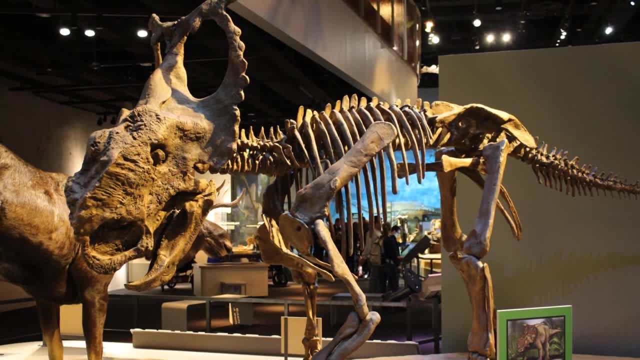 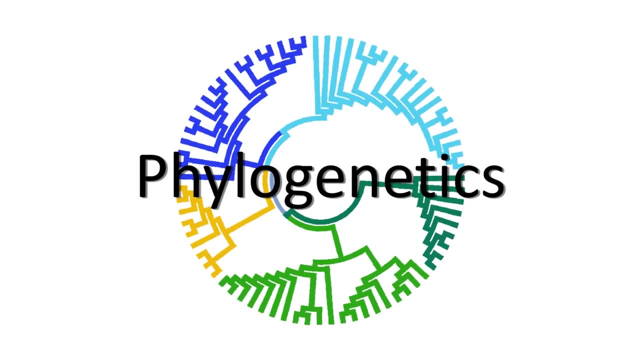 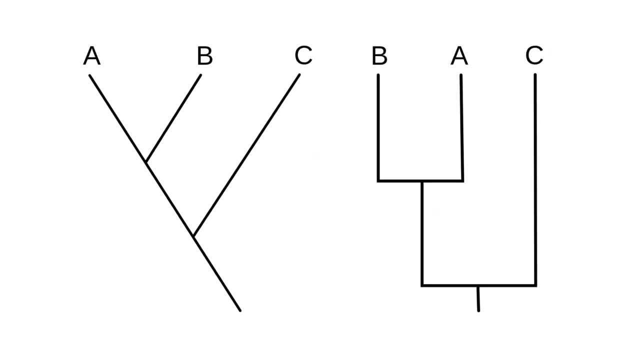 and would not involve the study of any soft tissues. Then there's phylogenetics, or phylogeny. This refers to the evolution of a group of organisms and is the area of study concerned with working out relationships and evolutionary history. A phylogenetic tree or a cladogram can be constructed from analysing the similarities. 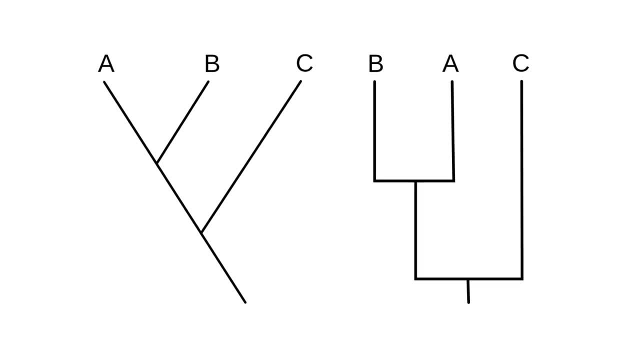 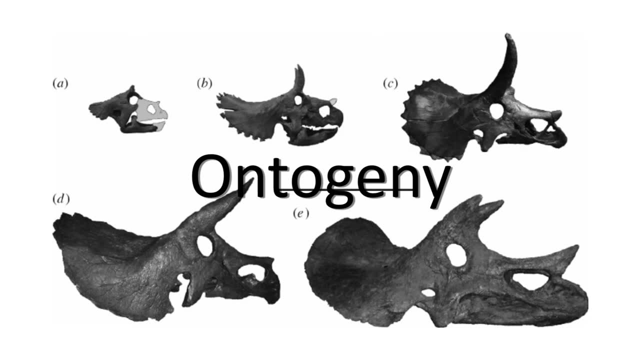 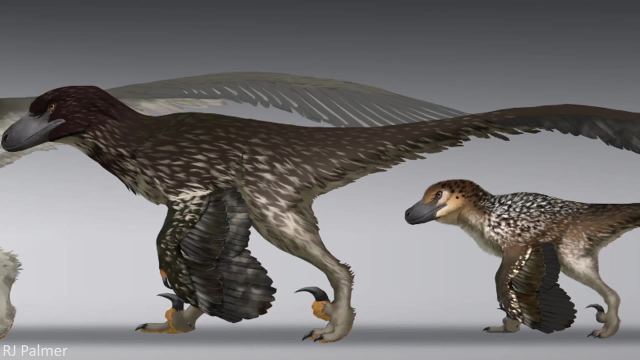 and differences in the morphology of extinct organisms, as well as the genetics of living creatures. Next we come to ontogeny, which I sometimes used to mix up with osteology, but it's pretty different. Ontogeny is the study of how an individual organism changes as it grows older, and so in paleontology you could see it. 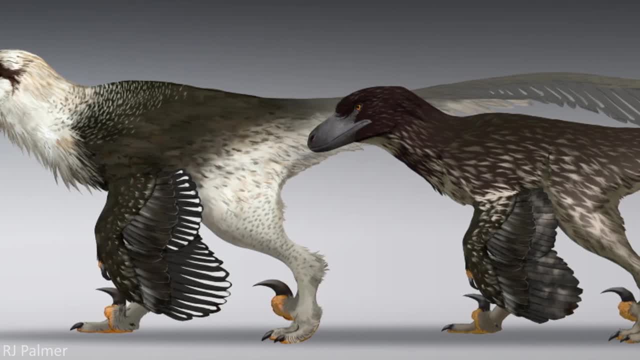 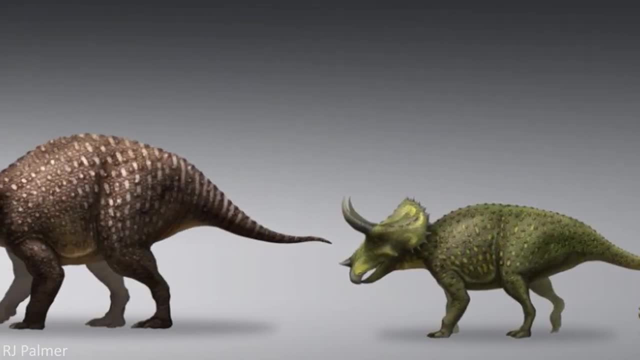 being discussed in paleontology as a whole and vice versa. In other words, photography is not just papers describing specimens of prehistoric animals that may not have reached full maturity at the time of death. Ontogenetic development can radically change the appearance of an 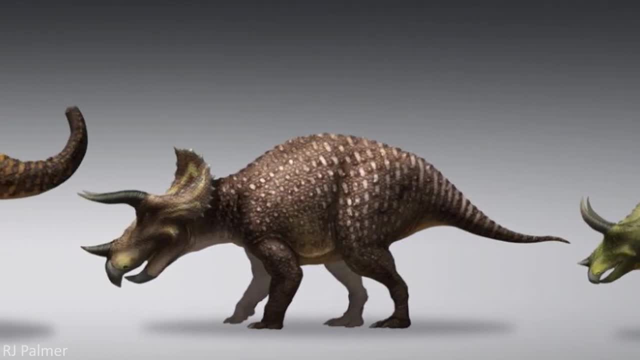 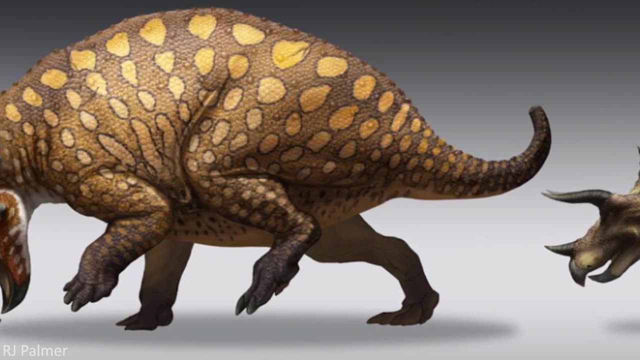 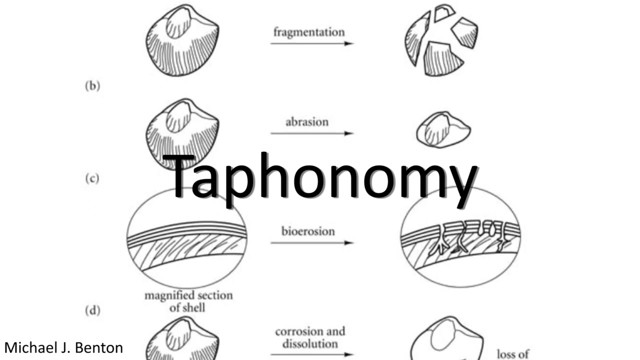 animal, and it's therefore sometimes difficult to identify a fossil as the same species as another older individual, especially when just a few fragmentary bones are known. so ontogeny is crucial to understand. Taphonomy is another particularly important field of study within paleontology, as it 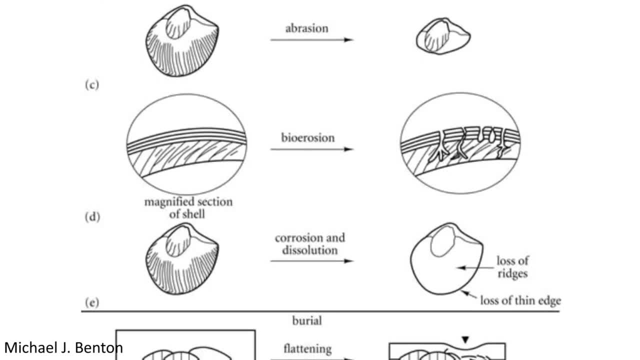 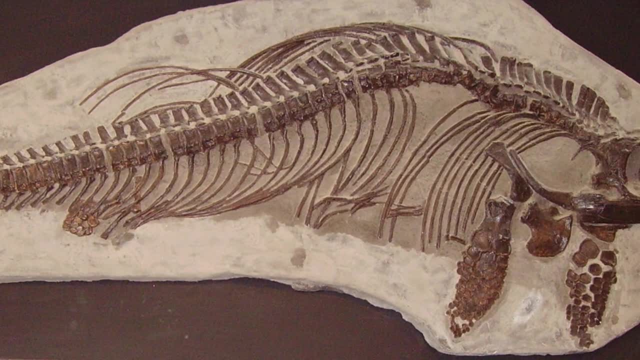 looks at the processes that affect an organism in the time between their death and their fossilisation, as well as any subsequent events that affect the fossil once it's in the ground. Taphonomy therefore allows paleontologists to understand why a certain fossil might be. 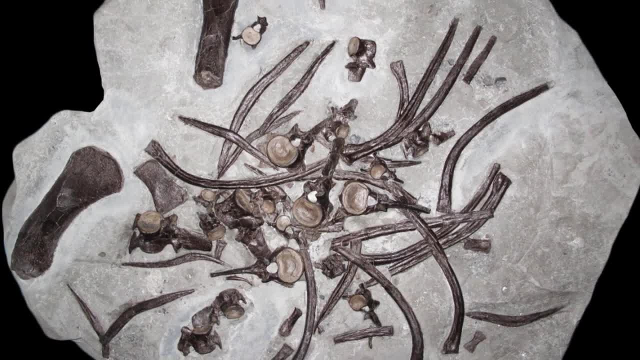 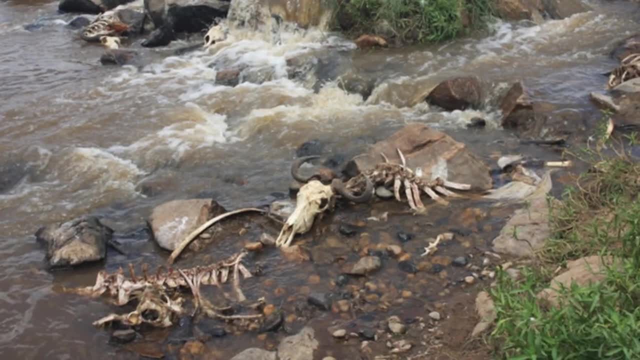 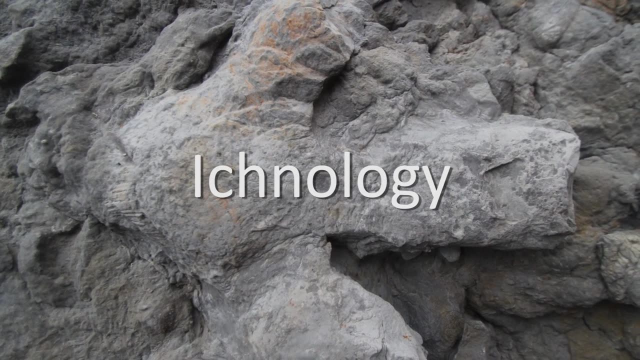 very complete and articulated, or why it is highly disarticulated and poorly preserved. It takes into consideration events such as scavenging, transportation, deposition and the physical processes that occur in rocks. There's also the field of ichthnology, which is the study of trace fossils. These fossils include things: 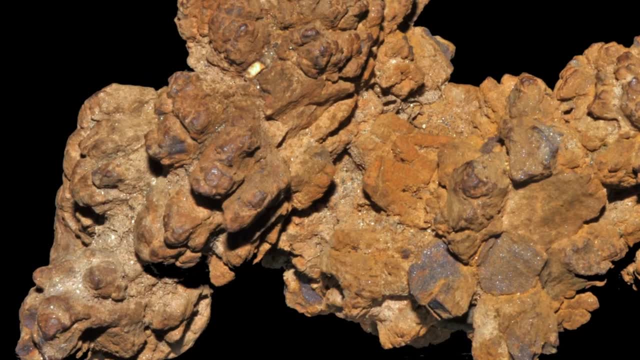 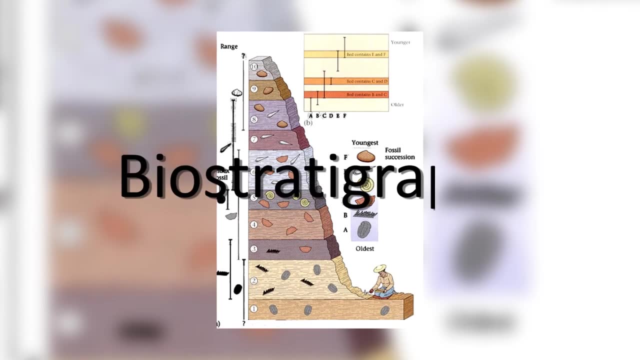 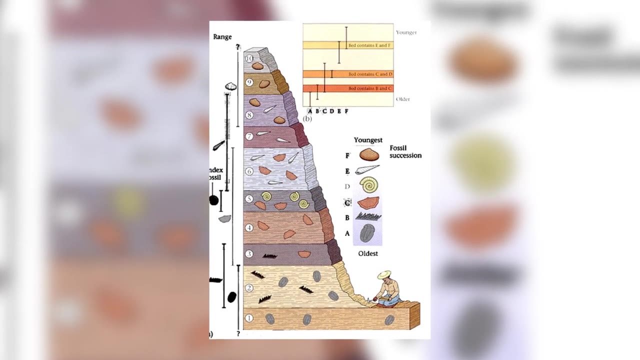 such as footprints, preserved burrows and coprolites, and they grant an especially valuable insight into prehistoric animal behaviour. Finally, you might come across biostratigraphy. This is basically the relative dating of rock formations using the fossils found within them, and it's, of course, important for understanding. 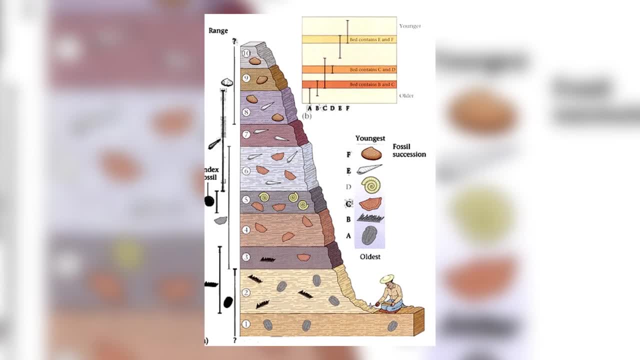 what sort of organisms lived at the same time as one another in the past. There are some common index fossils that are found in the past, such as the one found in the late 19th century. There are other examples that prove useful in dating using biostratigraphy, as they're. 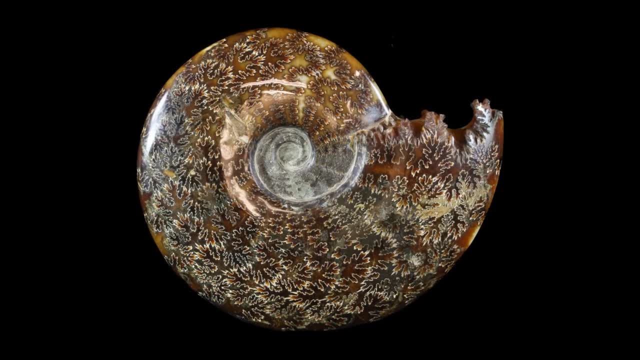 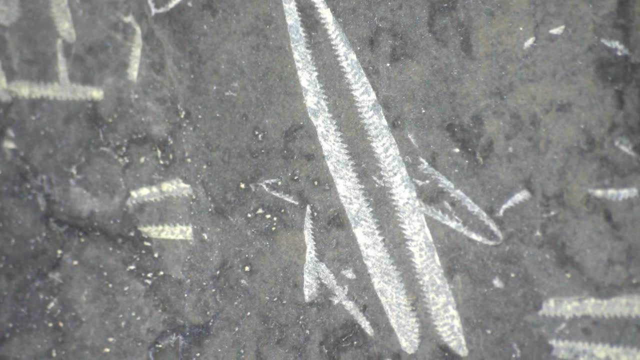 relatively abundant and evolve fairly rapidly, with certain species only being around for certain parts of the Earth's history. Ammonites, trilobites and graptolites are some examples of these. There are probably more sub-branches and research topics within paleontology that you'll encounter. 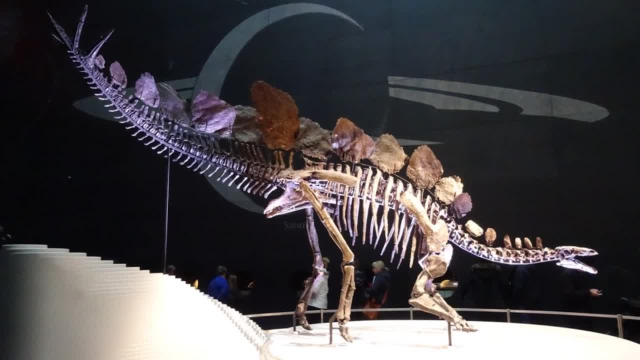 but these are some of the most basic ones that are pretty important to know Right next we're going to go through some of the basics of anatomy orientation. This is fairly simple, but it's not as simple as you might think it would be if you didn't. 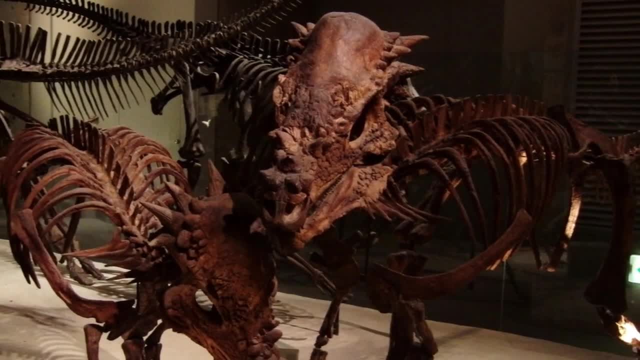 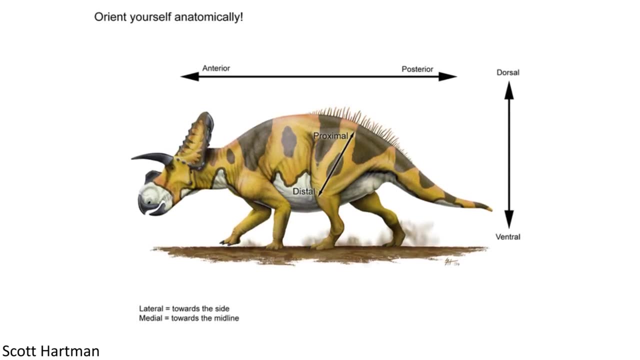 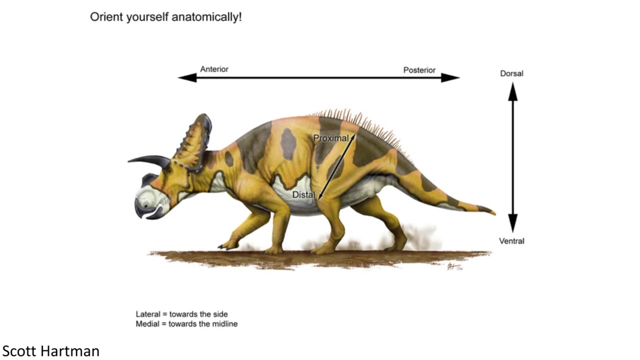 know There are a few technical terms for the directions you're talking about and it can get a little more confusing when they start to be combined together. First there's anterior and posterior. Very easy to understand: Anterior just means towards the front or the head, posterior means towards the back or the tail. 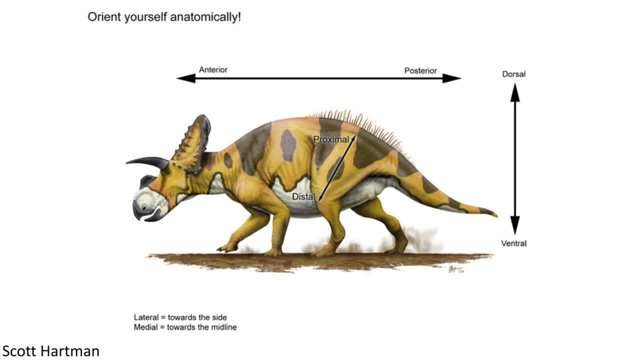 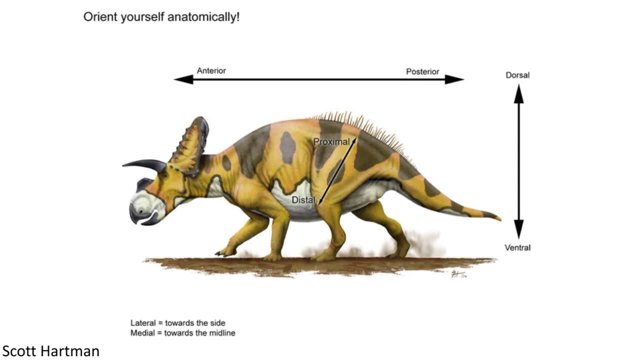 Dorsal and ventral are pretty simple too, with dorsal referring to the upper region and ventral to the lower region. Next there's medial meaning towards the midline and lateral meaning away from the midline and lateral meaning towards the midline. So I think this: 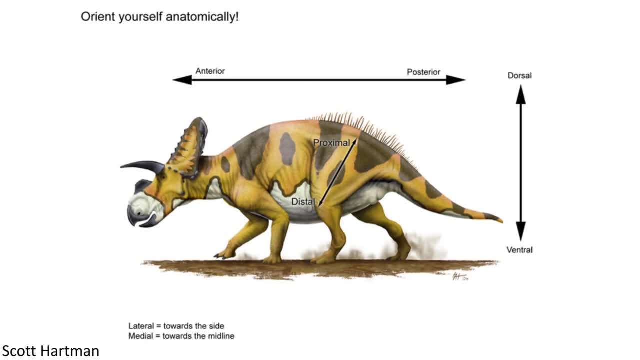 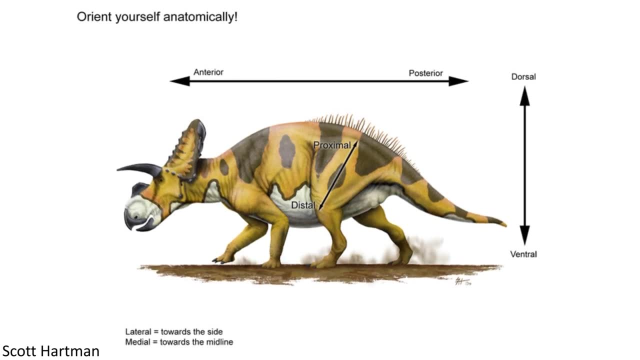 means away from the midline and towards the side. Then there's also proximal and distal, which convey placement in relation to the core of the body. Proximal means something is towards the main body mass, and distal means it is. 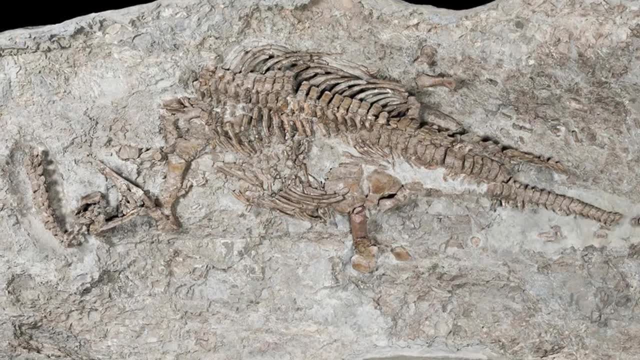 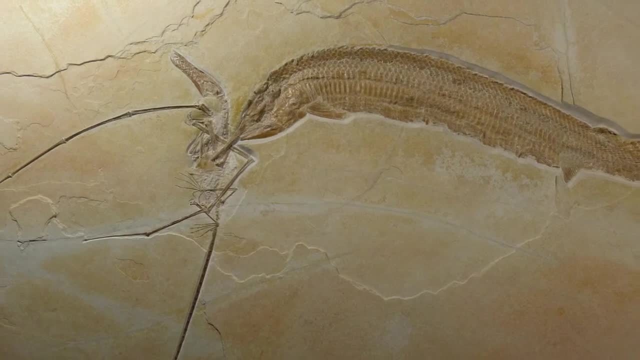 away from it. These words are all very useful in communicating how a bit of anatomy, such as a fossil bone, is positioned in relation to the rest of the organism, But, as I mentioned, you can get even more precise by combining these terms together. 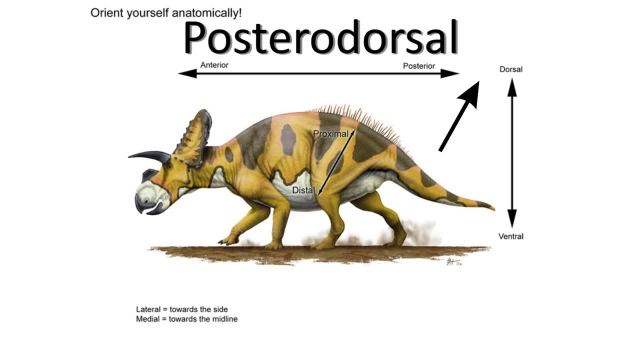 For example…. Prosteradorsal would refer to the back part of the upper region of an organism or part of an organism. Additionally, if something is said to be compressed dorsal-ventrally, that means it's flattened along the lower and upper sides. 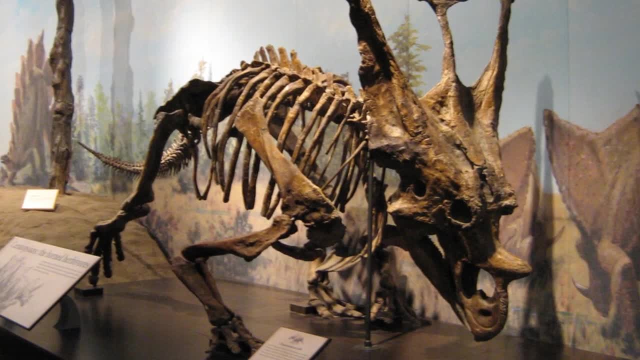 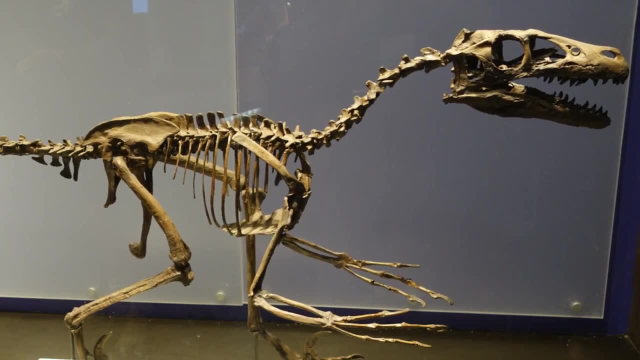 So it's not too complicated to understand what's being discussed with these terms, but it can seem unclear if you haven't encountered them before. Now, skeletons are a big part of vertebrate paleontology and therefore it's important to know the names of the main bones you will likely come across, For example, the main bone. of the vertebrate paleontology would be the vertebrae. On the other hand, a large chunk of bone is considered a vertebrate paleontology as well, And it's important to know the names of the main bones you will likely come across. 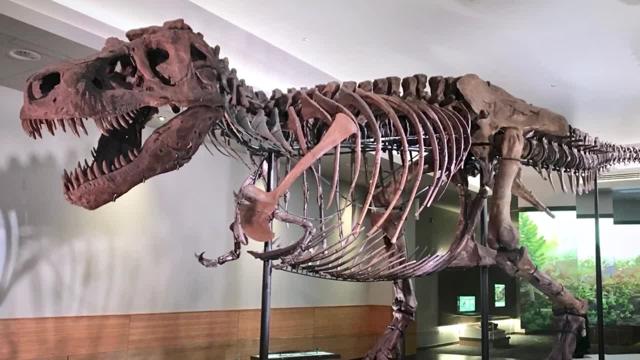 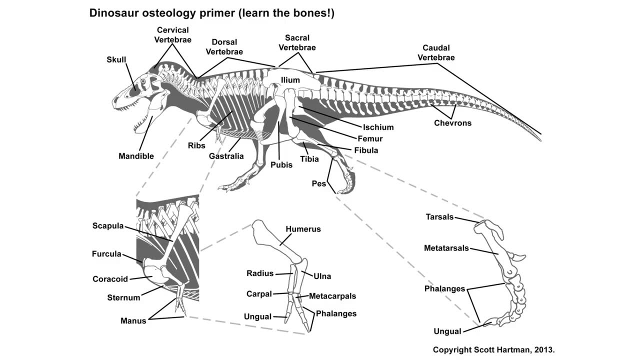 across. For this part, we're going to be using the example of a Tyrannosaurus. however, the exact bone anatomy does differ between animal groups. T-Rex is a pretty good model for our purposes, though, and Scott Hartman, renowned for his excellent skeletal reconstructions, has made. 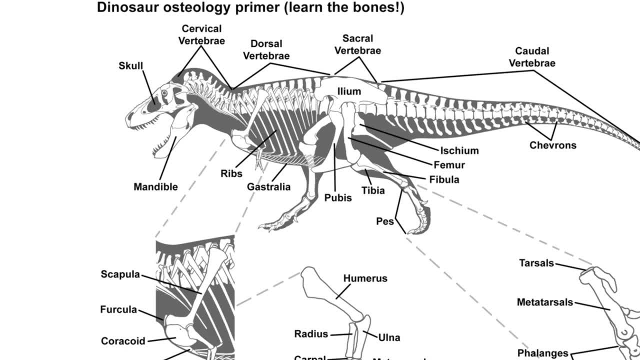 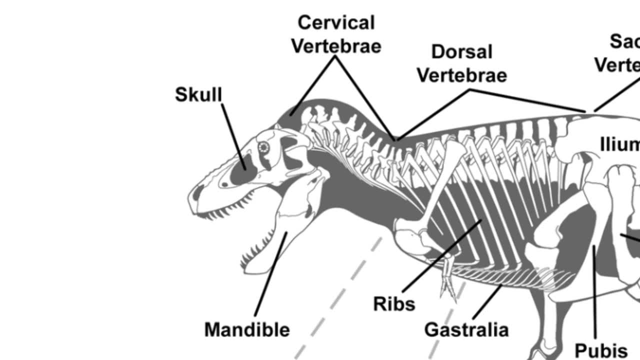 a wonderful guide to the elements that make up this creature. Okay, so, obviously, first there's the skull and the mandible, although these are actually made up of several fused bones that we'll get into later. The skull is attached to the anterior-most part of the vertebral column. 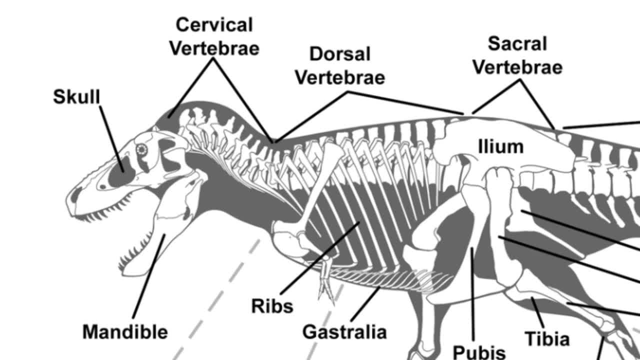 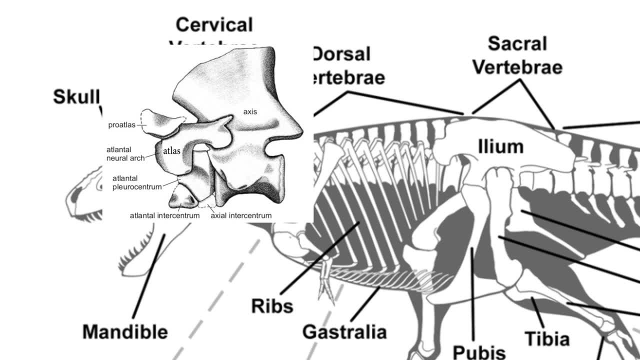 which is composed of bones called the cervical vertebrae, basically the neck bones. The first two of the cervical vertebrae have particular names and these are the atlas and the axis Posterior to the cervical vertebrae are the dorsal vertebrae, and behind them are the sacral 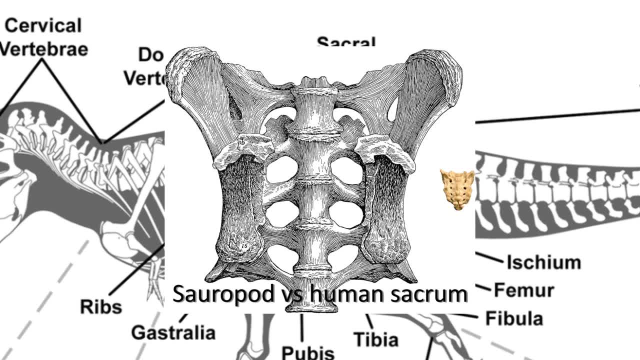 vertebrae, The sacral vertebrae, are interesting as they're all fused together and attached to the ilia or hip bones either side of them. The fused mass of sacral vertebrae is also referred to as the sacrum The most posterior. 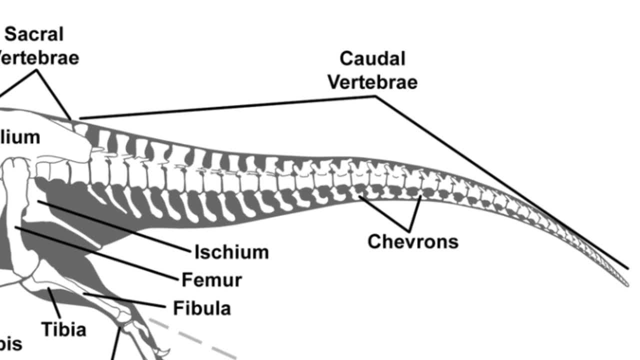 vertebrae are the caudal vertebrae, and these make up the tails of many vertebrates. Underneath or on the ventral surface of the caudal vertebrae are a series of bones called chevrons, which would 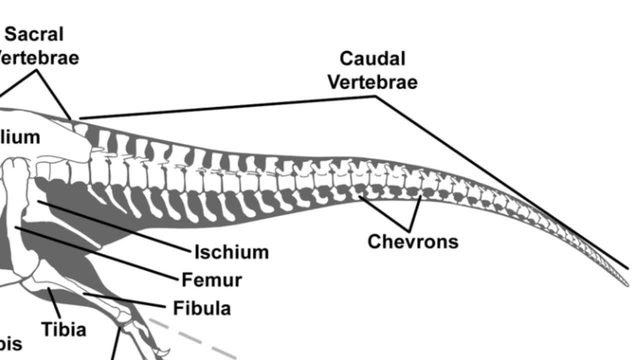 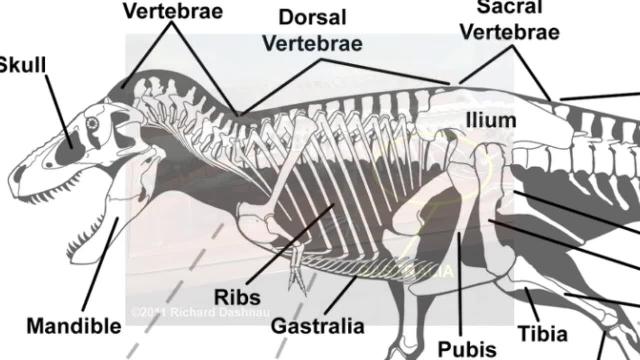 have contained blood vessels running through the gap in them in life. Attached to the dorsal vertebrae are the ribs, and underneath these are the gastralia or belly ribs. These structures can also be seen in the sacral vertebrae and these are the dorsal vertebrae. The dorsal vertebrae are: 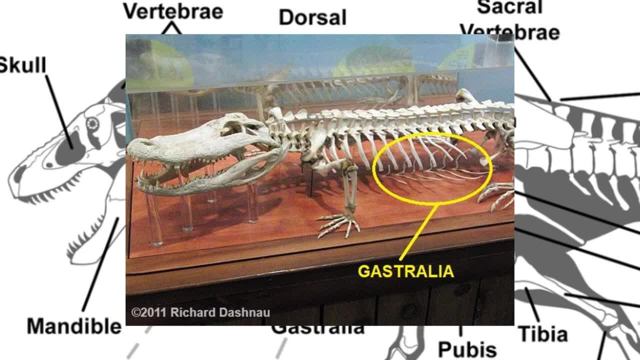 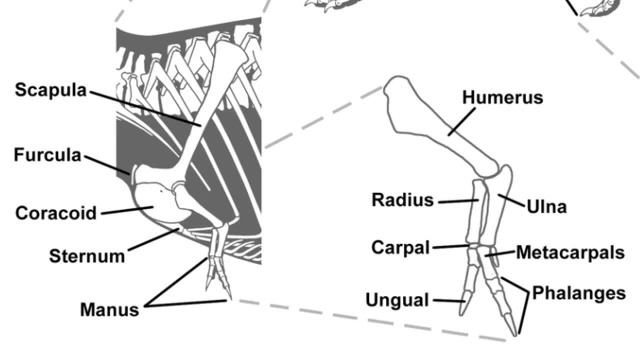 seen in modern crocodilians, as well as in various other extinct groups such as pterosaurs. Moving to the limbs, the general plan of the forelimb consists of the scapula and coracoid together making up the shoulder girdle and, below these, the humerus radius and ulna. 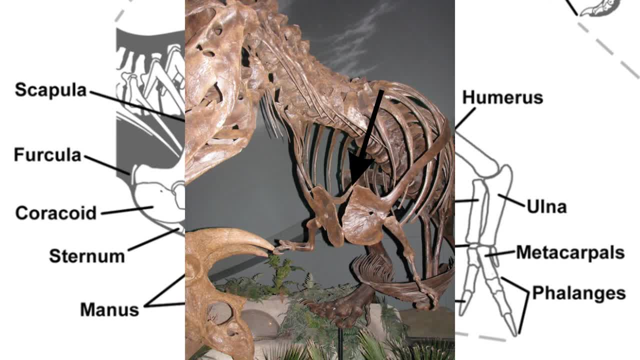 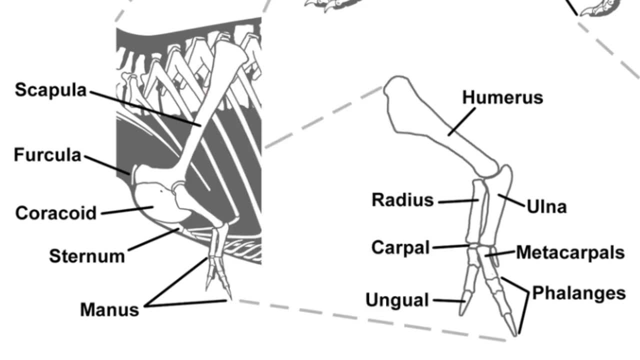 and the bones of the hands. In some theropod dinosaurs there's additionally a furcula in the chest region, also known as the wishbone, which is present in modern birds. The bones of the hands, or marnus, are the carpals, metacarpals and the cartilaginous. The cartilaginous. 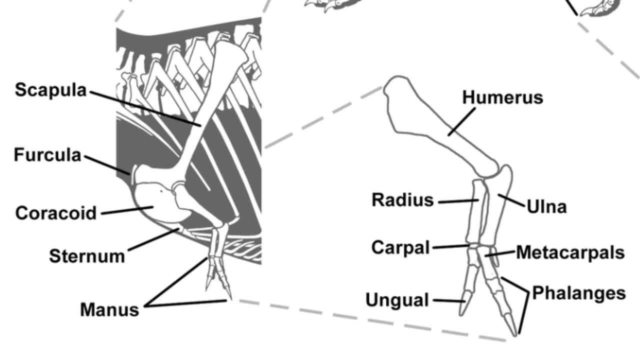 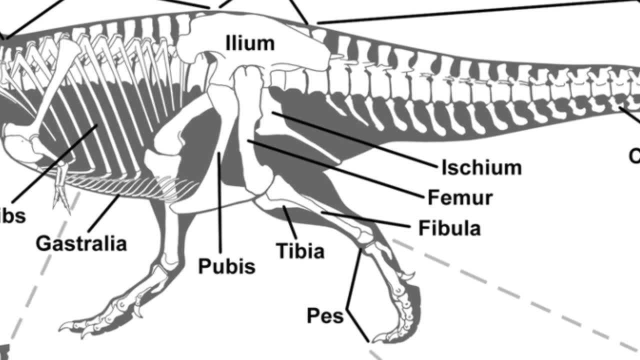 bones are the metacarpals phalanges and sometimes unguls, which are modified distal phalanges that form claws. The hindlimbs and pelvic girdle are next, with the hip being composed of three bones: the ilium at the top and the ischium and pubis underneath. 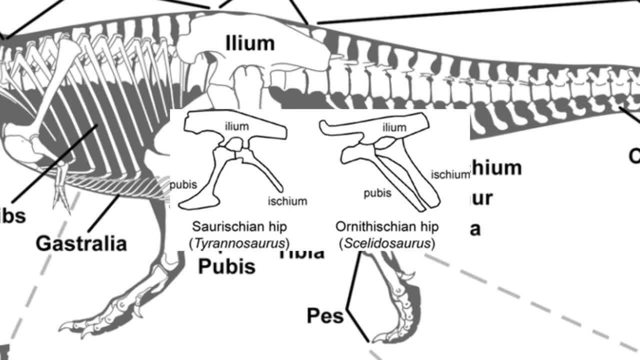 The positioning of the pubis, as you may know, has been used as one of the main distinctions between the traditional two groupings of dinosaurs: ornithischians and saurischians, with ornithischians having much of the pubis pointing posteriorly and marnus having much of the pubis pointing. 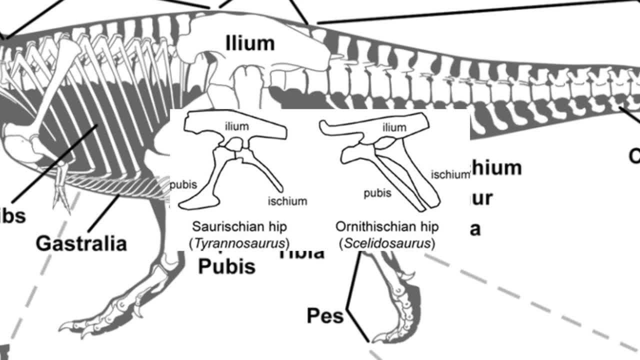 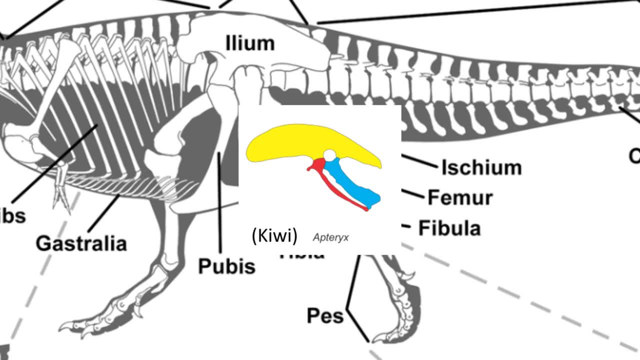 posteriorly, and most saurischians having a pubis that projects more towards the front. Birds and their close theropod relatives are an exception to this, however, and of course the whole classification of major dinosaur groupings is something of a complicated debate. 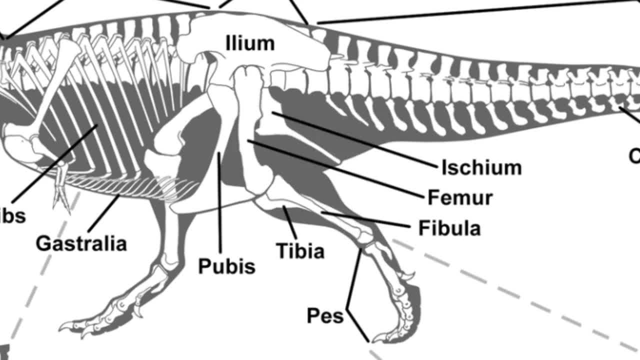 anyway, Attached to the pelvic girdle at a socket called the acetabulum is the femur, and below that the tibia and fibula. Non-avian dinosaurs did not have a kneecap, known as a patella, like us mammals. 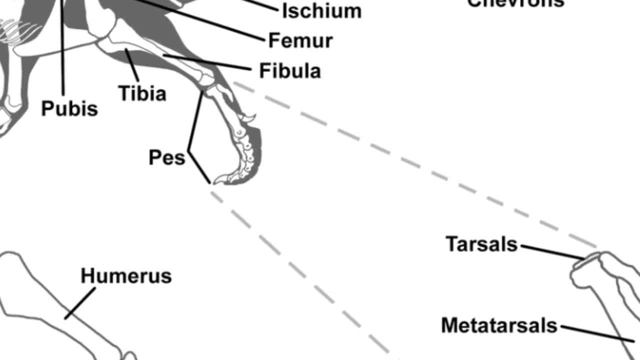 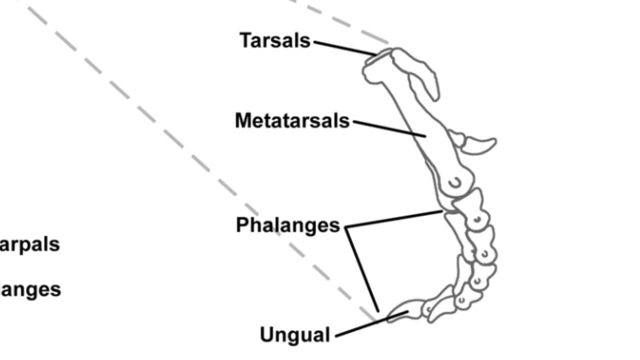 The hind foot, technically called the pes, has a similar composition to the hand. however, some of the bones have different names. Instead of carpals and metacarpals, there are tarsals and metatarsals, but there are still phalanges and some modified unguls. 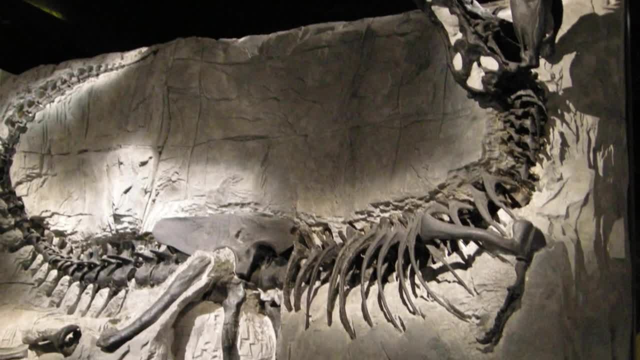 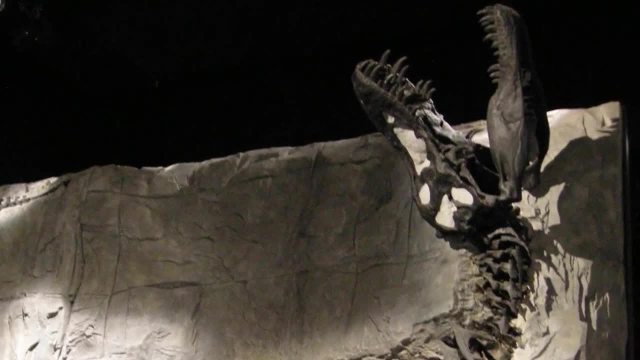 So that's a brief overview of the general skeleton of a tyrannosaur, but keep in mind that different animals have all sorts of different bones, and so there will be some terms that were not mentioned here. Now, the skull anatomy is also useful to know in paleontology. 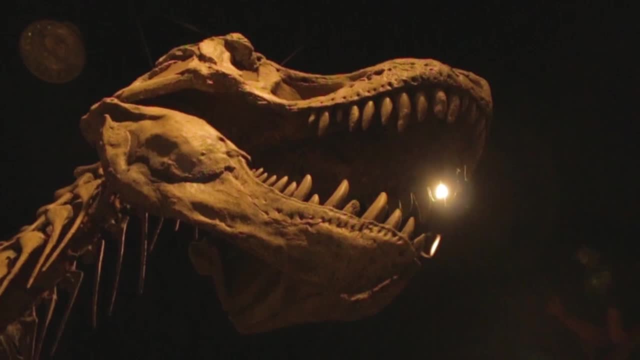 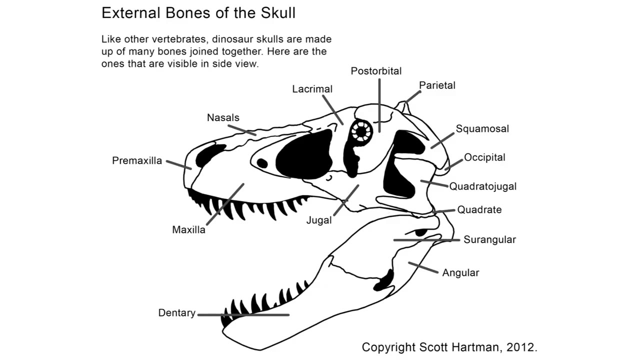 Since, as I said before, they are made up of many bones all fused together, and there are also names for the various holes in the skull. Again, I'll here be using Scott Hartman's fantastic labelled reconstructions of t-rex bones. 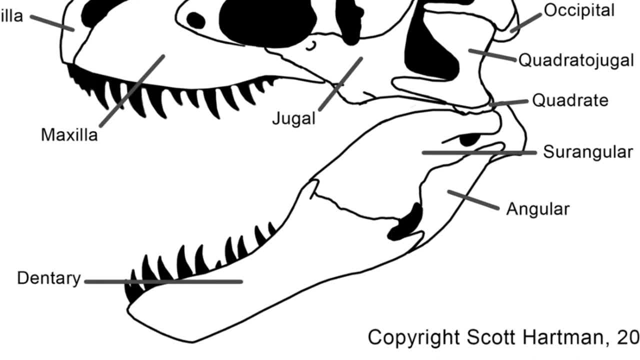 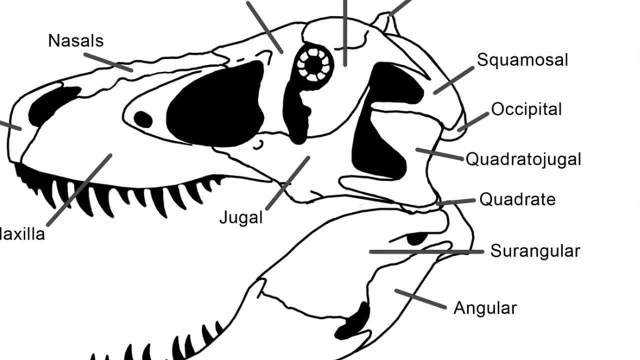 The mandible of Tyrannosaurus is comprised of the dentary as well as the angular and the serangular Part of the jaw joint is made from the quadrate which you can see here attaches to the quadrata jugule. The rest of the bone names are fairly self-explanatory. 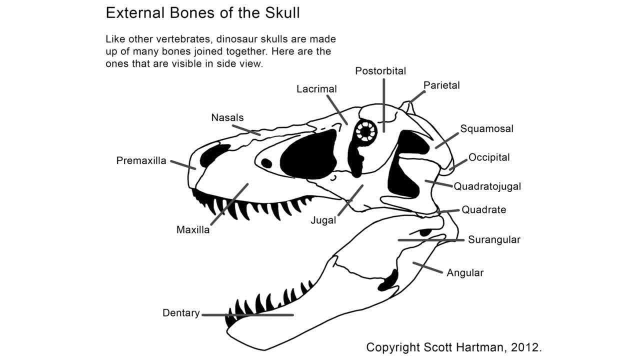 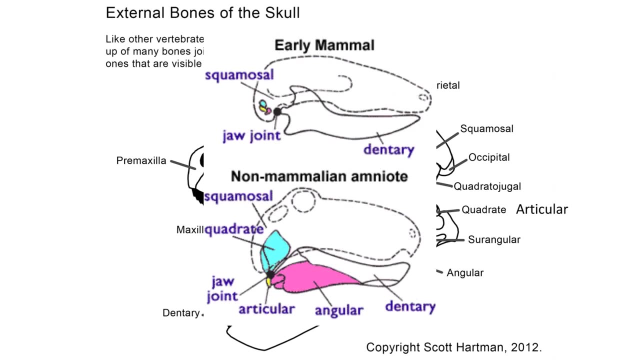 and just make up the different regions of the animal's skull. Obviously, the placement and shape of the bones vary hugely between evolutionary groups and it's also worth pointing out that, interestingly, the quadrate and another bone not shown in this diagram, the articular, actually migrated into the skull in mammals to become the auditory ossicles. 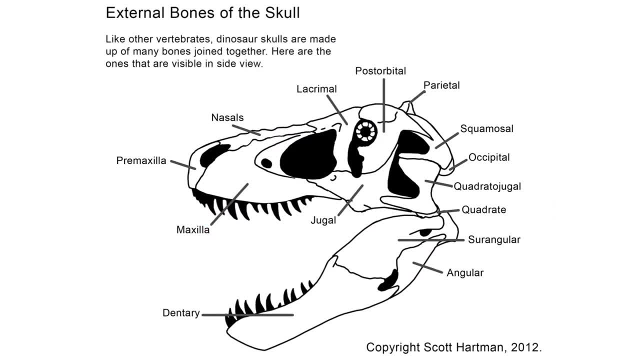 the middle ear bones we use for hearing. So if you come across names such as maxilla, premaxilla, jugule, lacrimal, and so on, this diagram will be very useful in figuring out which skull bone is being talked about There. 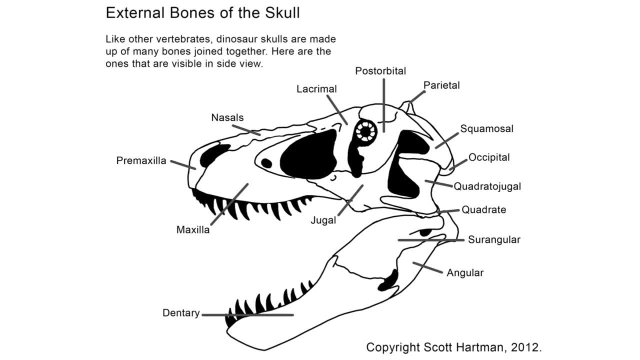 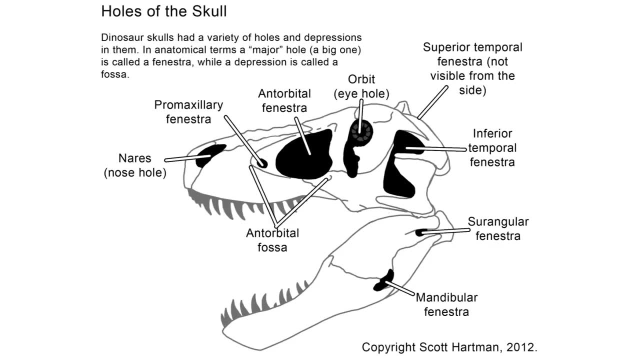 are links to these images down in the description, so be sure to use them if you think they'll be useful. They certainly were for me. But what about the spaces between the bones? Well, Scott Hartman has an easily understood guide to those as well. 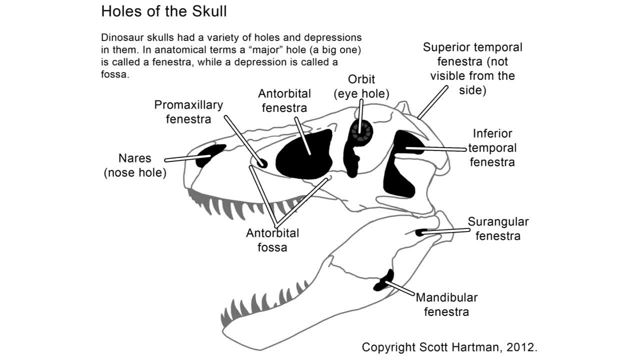 The largest holes in the skull are technically termed fenestrae, the singular being fenestra, which comes from the latin word for window, whereas a smaller depression in the bone surface is known as a fossa, Not to be confused with the Madagascan carnivorum. 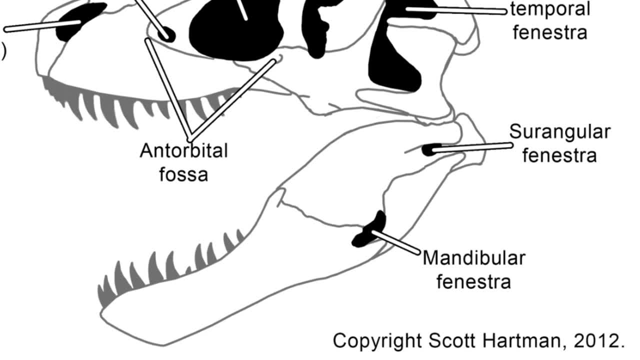 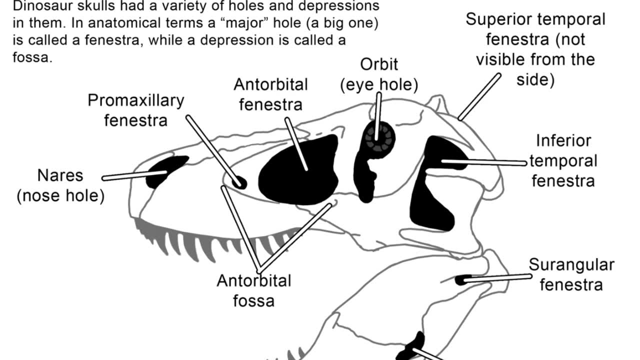 The mandible of T rex has two major holes in it: the mandibular fenestra and the serangular fenestra. There are then quite a few openings in the rest of the skull with the nares orbit and several fenestrae. 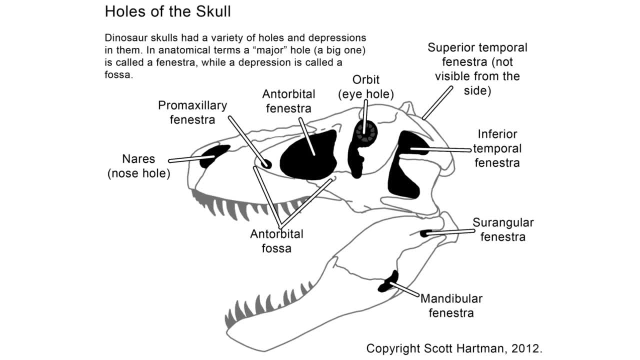 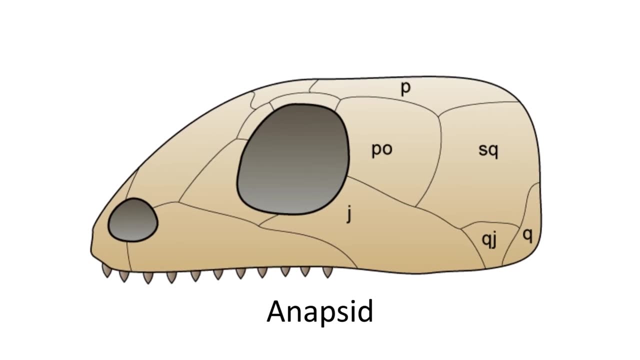 Now, the number of fenestrae that an animal possesses is quite significant in the classification of the organism, with different groups being given different names depending on the holes in their skulls Considered, the most basic condition in vertebrate skulls is that where there are no fenestrae in the skull at all, Organisms with this skull 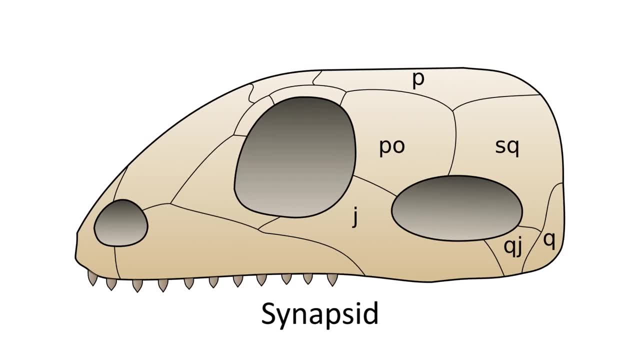 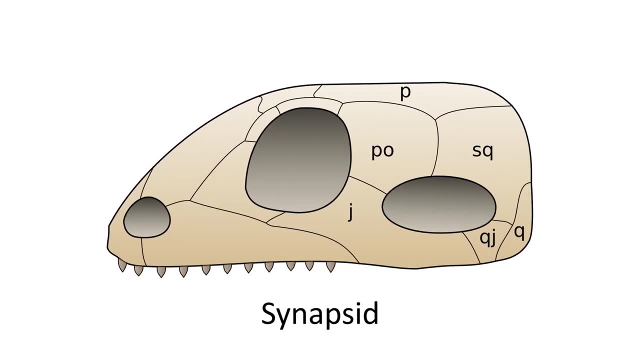 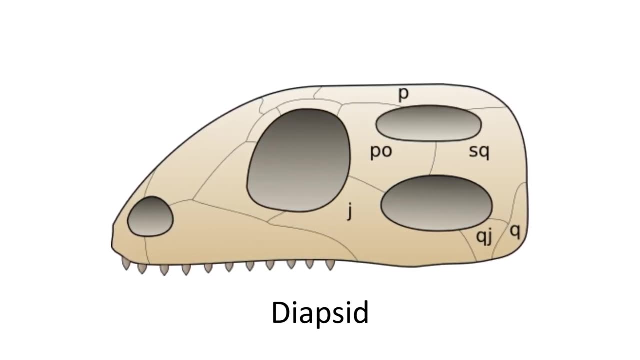 morphology, are termed anapsids. Next are the vertebrates with one temporal fenestra behind the orbit, the synapsids, which include mammals and some lineages closely related to mammals. Then there's the diapsids, containing many reptiles such as crocodilians, lizards, snakes, turtles and birds. The diapsid. 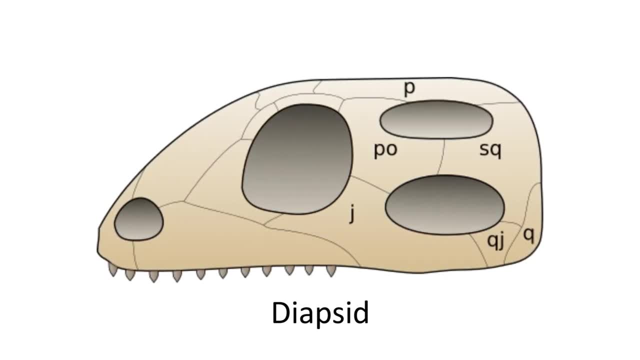 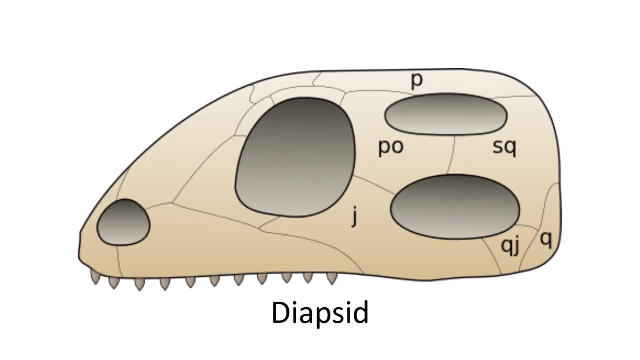 condition is a skull that possesses two openings behind the eye socket. however, due to the changes over time, there are some diapsids with only one or no fenestrae posterior to the orbit, but they're still classified within diapsida. Now there's also a grouping termed the uriapsids, which have a single fenestra behind the eye. 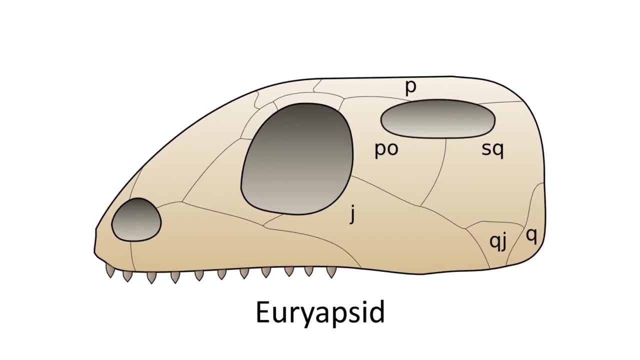 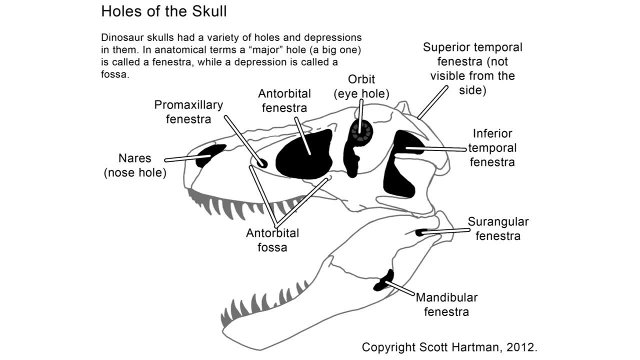 placed high on the skull. however, like the anapsids, they have been found to be an unnatural grouping of animals that should, in fact, probably be classed as diapsids. Dinosaurs such as this t-rex are themselves diapsids. as you can see, they have both an. 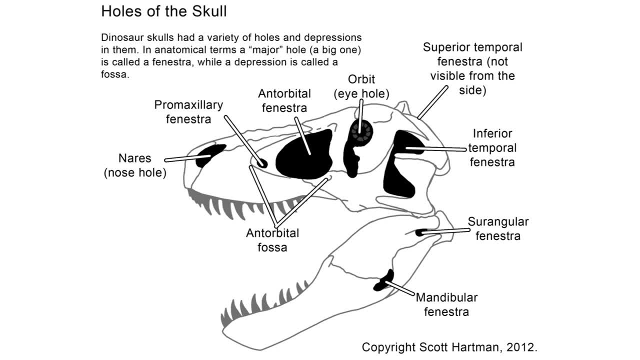 inferior temporal fenestra and an anapsid. They additionally have antorbital and promaxillary fenestrae in front of the eye sockets as well. Okay, well, hopefully this quick introduction to osteology has been useful and, as I said, 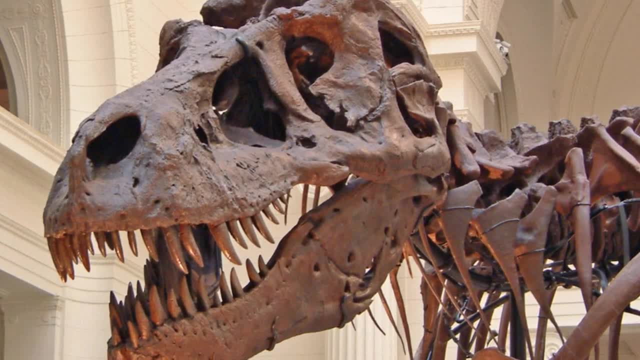 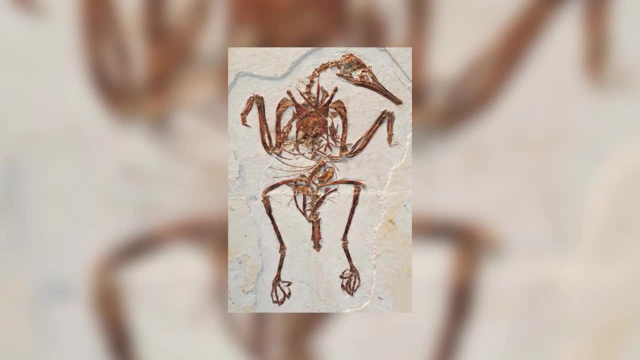 I'll link to Scott Hartman's diagrams in the description so you can use them more if you would like to. Next we're onto a brief overview of some evolutionary terms that could come in quite handy when learning about paleontology. Of course, understanding evolution is pretty. 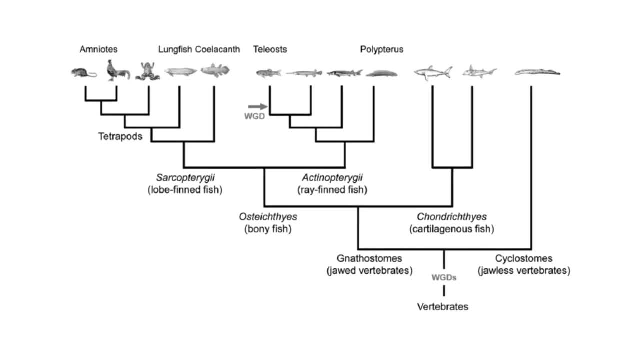 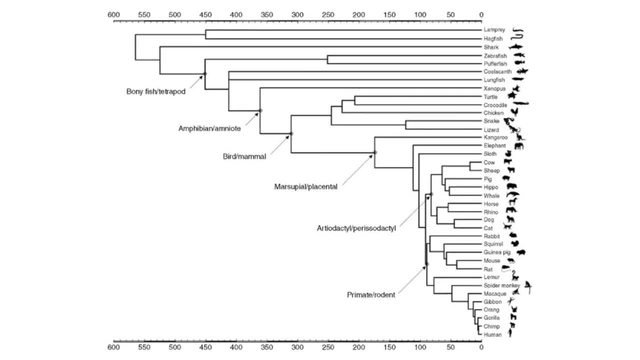 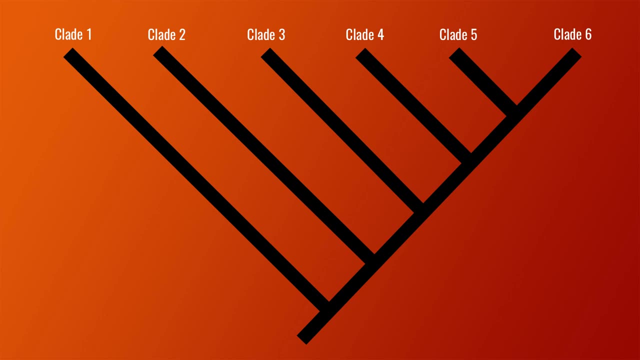 integral to all of biology, But particularly so in this science, as we're constantly dealing with organisms from a variety of branches across the evolutionary tree, and finding out where they belong on it can help us infer a great deal about these extinct beings. Okay, so you've probably seen one of these before, like an evolutionary tree, as I just 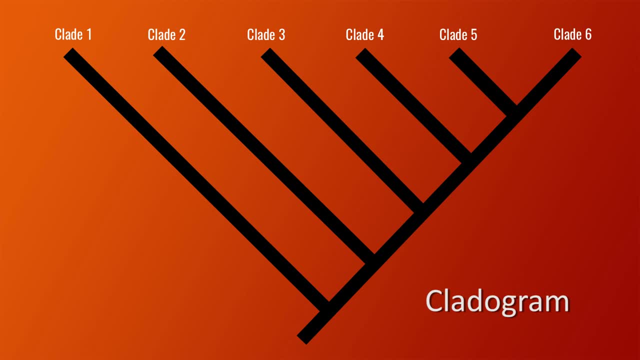 mentioned. Technically they are called cladograms, and they allow us to view how various organisms are related to one another. The evolutionary groupings of organisms are termed clades, and they're basically the same thing as groups such as classes, orders, families and so on. 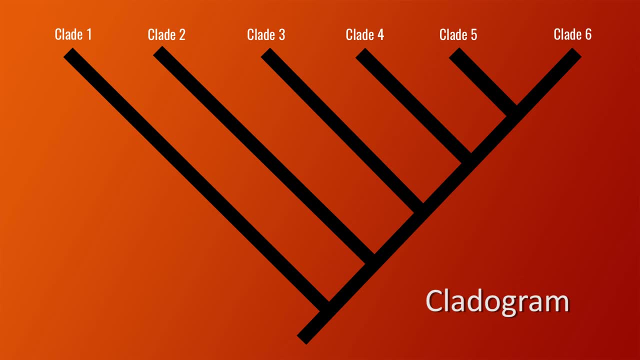 that are used in Linnaean classification. However, due to the huge number of groupings and complicated occurrence of evolution, paleontologists now usually just refer to every group as a clade. Cladograms are used to visualise these clades with lines representing different taxa branching. 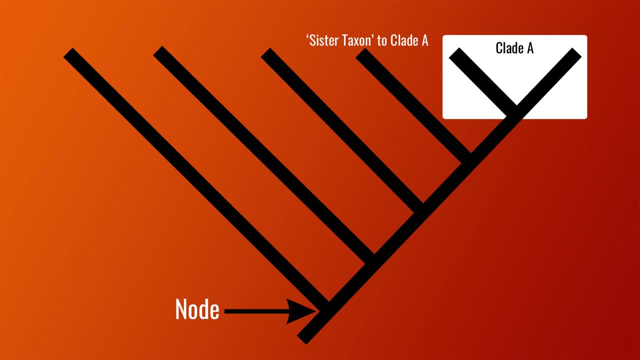 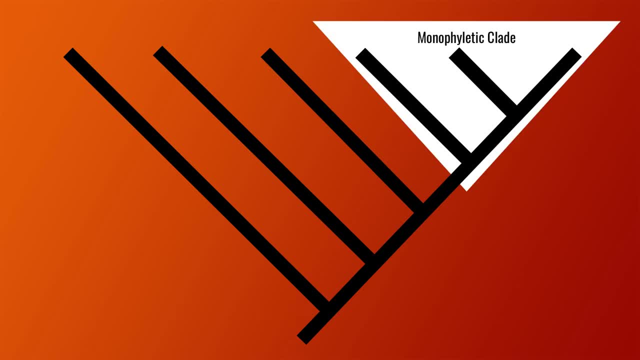 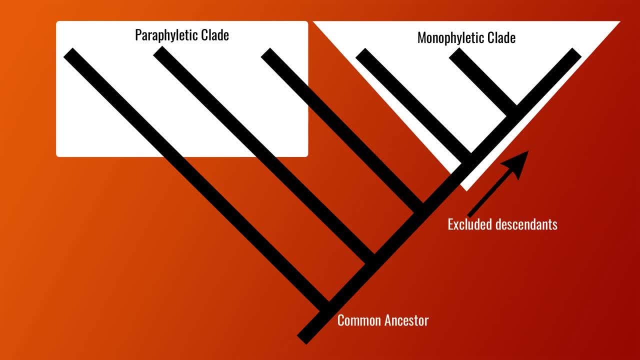 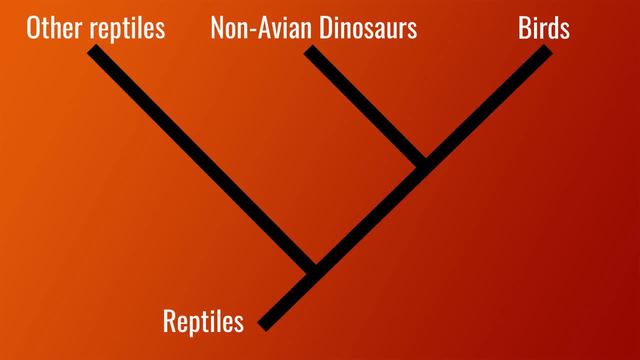 clade is an unnatural or artificial grouping, which is where the group has a common ancestor, but some descendants from this ancestor are excluded from the grouping. A good example of this is birds and reptiles, Since birds evolved from dinosaurs, which are reptiles. 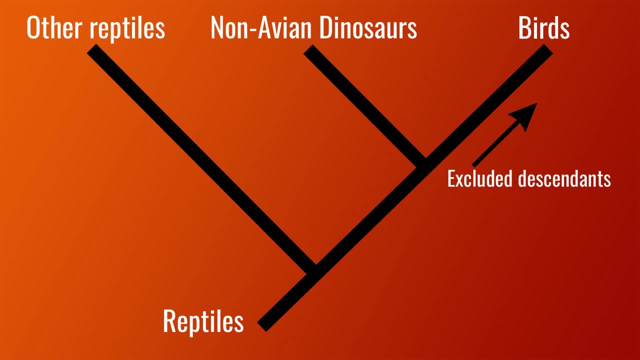 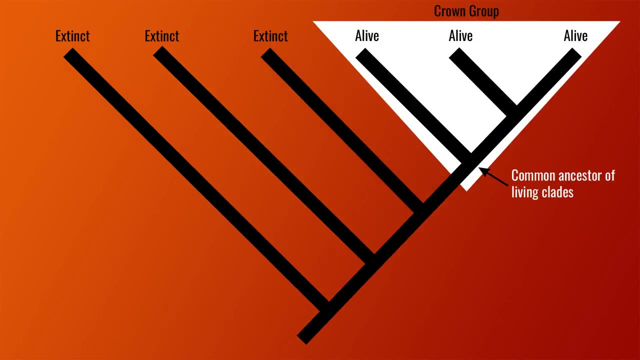 birds are reptiles. However, the usual definition of reptiles would not include birds, therefore making the clade Reptilia paraphyletic. Then there's also stem groups and crown groups. These aren't too complicated to understand. A crown group is just the clade containing the most recent common ancestor of all. currently, 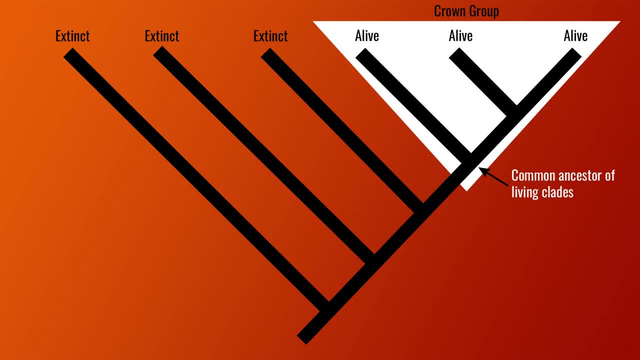 living species of a group of organisms and all the descendants arising from that ancestor. A stem group, therefore, is simply the extinct relatives of a crown group that are not themselves a part of the crown group. So this automatically makes stem groups paraphyletic, as I explained before, since they exclude a group Additionally. 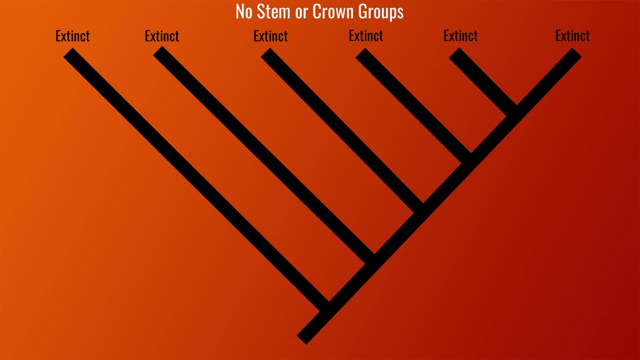 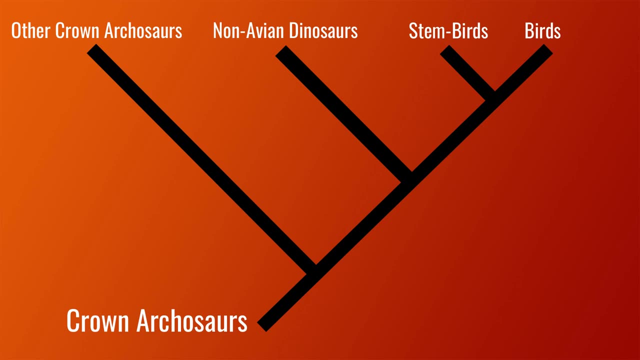 there can be no stem groups for a lineage that is already extinct. However, stem groups for some clades can be within the crown groups of larger clades. So, for example, stem birds are contained within crown archosaurs Right. so there is a lot of. 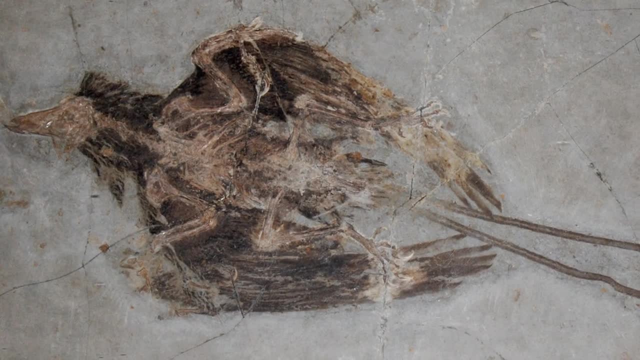 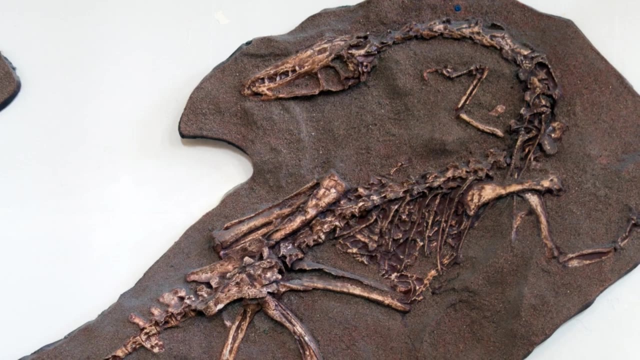 information to go through there and hopefully I've managed to explain it in an understandable way. There's definitely more to learn when it comes to phylogenetics and interpreting cladograms, but I think what I've gone over here is a pretty decent quick introduction. 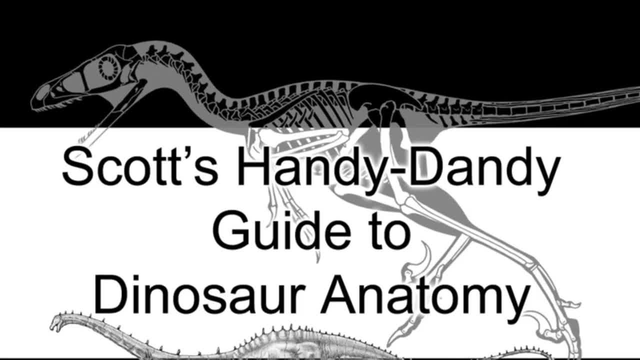 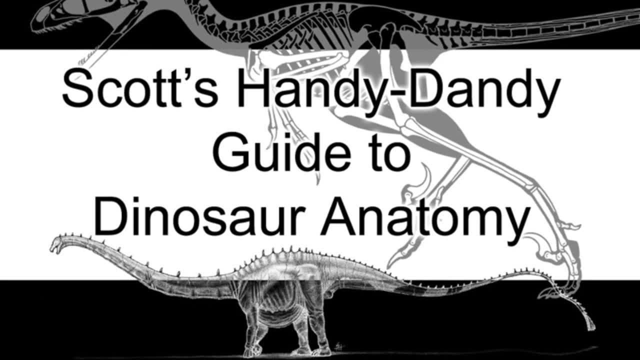 to the basic ideas in relation to paleontology, And hopefully this whole guide has been of some use to you. though I would recommend having a look at the anatomy guides I've posted the link to in the description too. There's even a guide to the musculature. 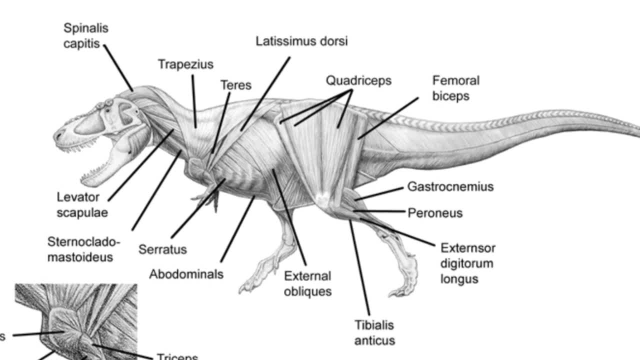 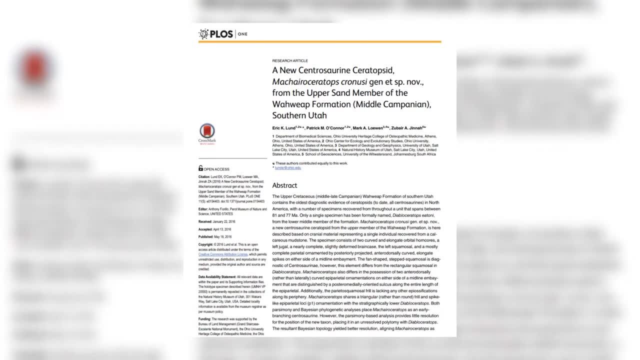 of dinosaurs, using T rex as an example, which I haven't included in this video. As I've already said, probably the best way to learn more about this science and to keep getting used to the technical terms used in it is to just read as many papers and 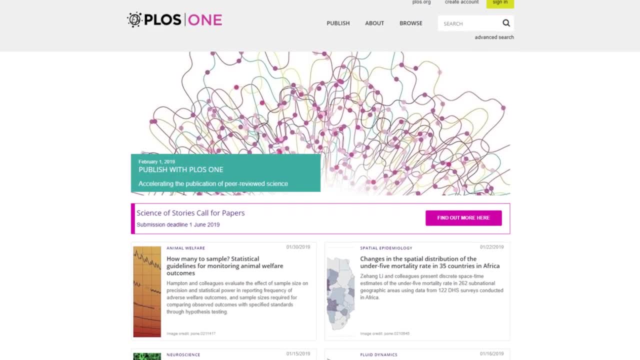 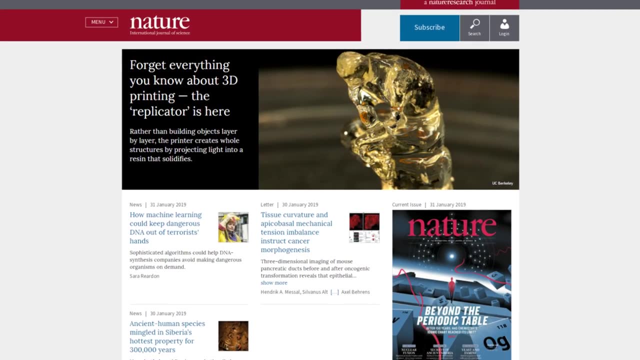 studies as you can. There are a great deal of free, open access papers available online, and sites such as PLOS ONE, PeerJ and Nature are good places to look, And even if the paper you're interested in isn't open access, there are ways to get around that. 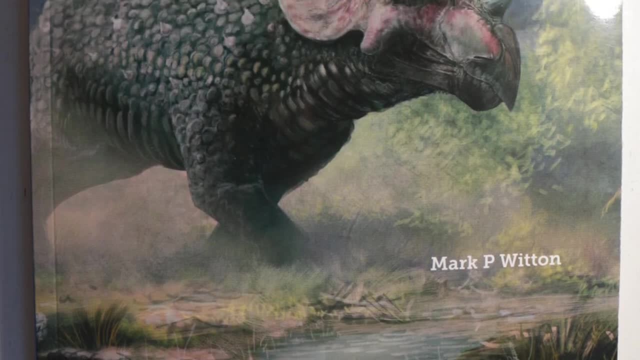 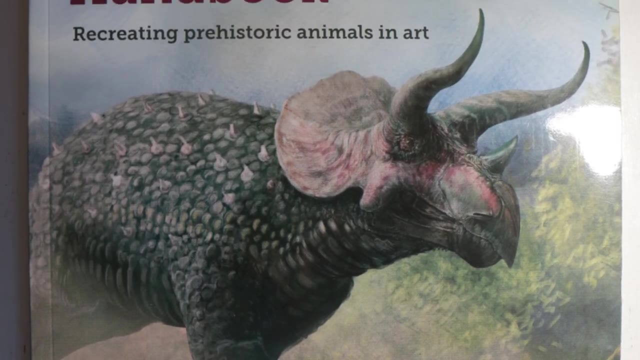 I should also mention that this video was partly inspired by paleontologist and paleoartist Mark Whitten's latest publication, The Paleoartist's Handbook, which has a great introduction to some of the essential technical terms used in paleontology, as well as diagrams showing 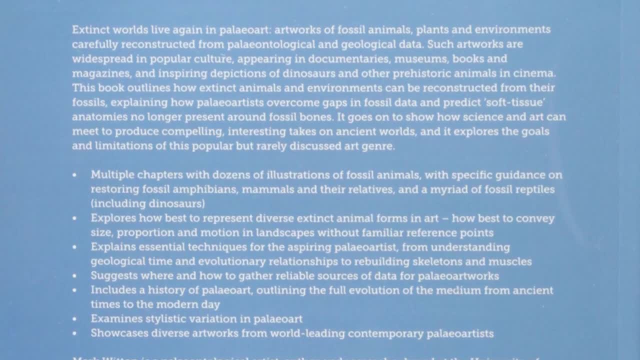 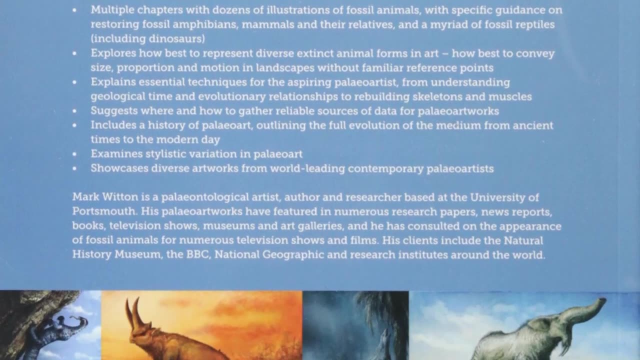 osteology and how to interpret cladograms. I would absolutely recommend getting this book if you can, especially if you're interested in creating your own paleoart or even if you just want to find out about the research and reconstruction processes involved in doing 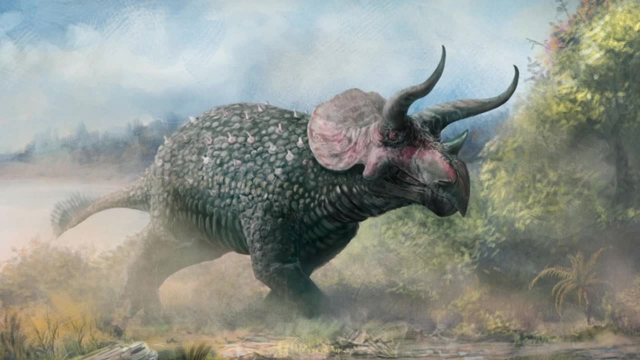 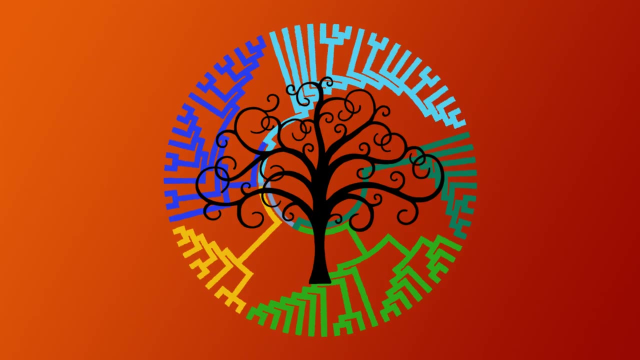 so, Anyway, this book gave me the idea of making a video as an introduction to paleontology, and I felt it might be helpful for some people, as it would have been for me. Well, I hope you enjoyed this video and learned something new, If you would like to find out. 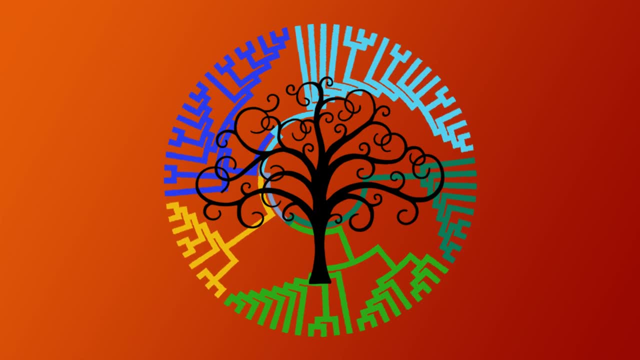 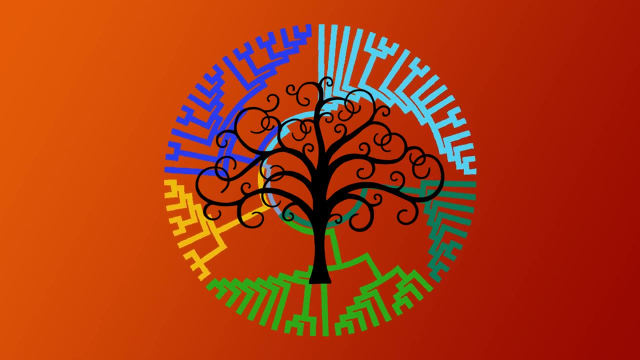 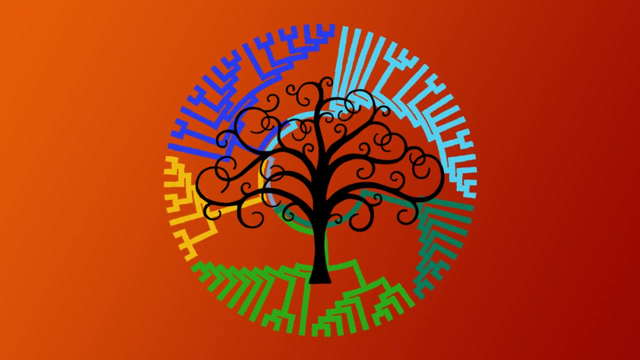 more about our world, its history and the wonderful life that surrounds us all. please feel free to subscribe to the channel if you think we deserve it and if you would like to see more from us. Subtitles by the Amaraorg community. 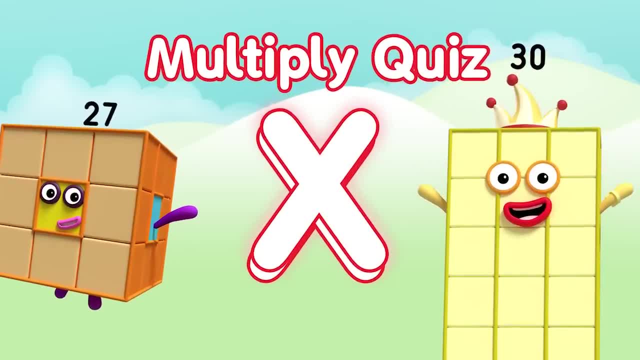 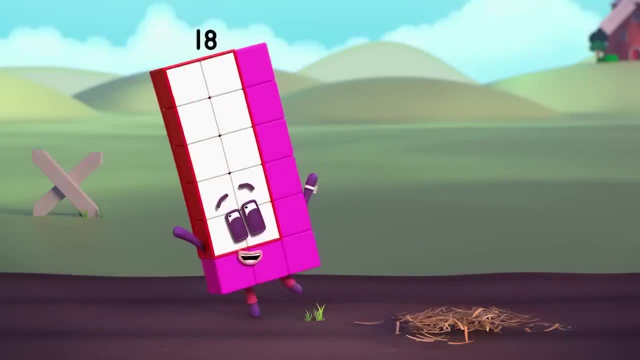 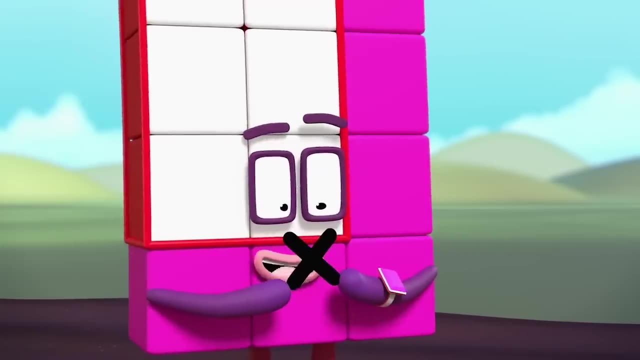 It's a sign, A sign that we need a new sign, A faster sign. We don't need all these Squash. We can add a number lots of times, Much faster with just one of these. I'll call it the times. 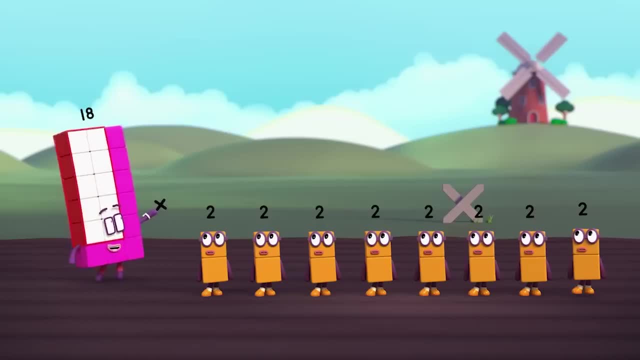 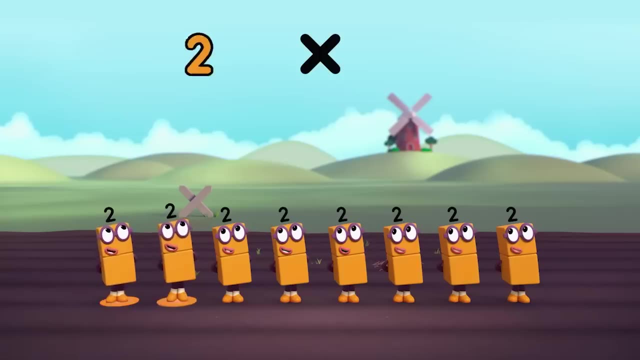 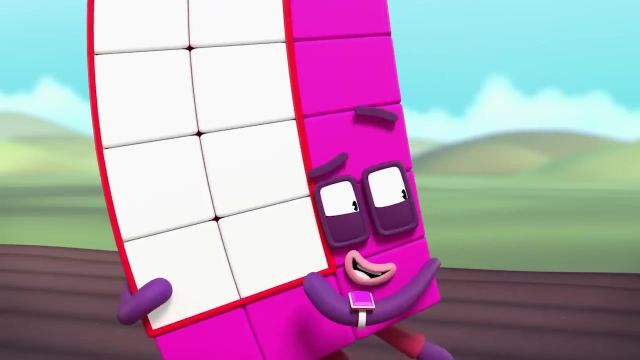 sign. I can use it to add something lots of times Super quickly. So how many twos are we adding? One, two, three, four, five, six, seven, eight. And remind me what are we adding again? Twos, Eight, lots of two On your marks. Get set, Go. Eight times two equals. 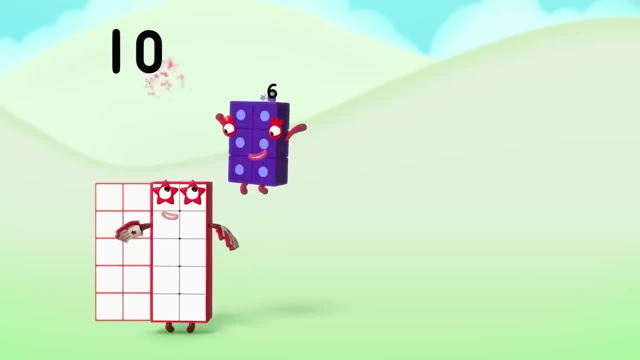 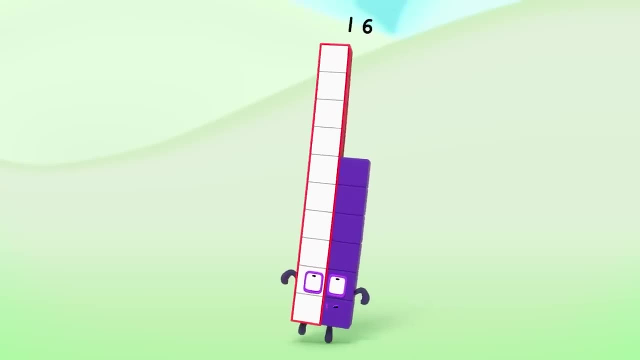 Sixteen, Ten plus six equals Sixteen. Oh, look, Here I am then. Well, that's nice, isn't it? Right, then Let's get on with it. See what shapes I can make. Yeah, Hmm, Ooh, Um. 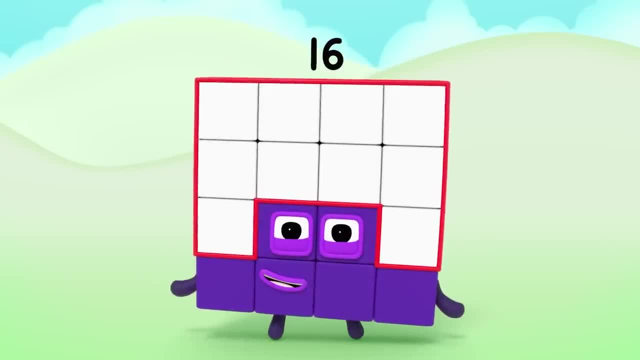 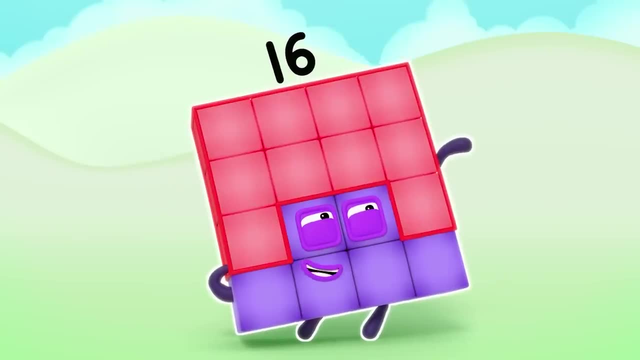 Aha, Oh, Oh, No, No way, I can't believe it. I'm so excited. Guess what I am? I am, I am, I'm 16.. And I am a squire, Wooh-ah, Right then, What do squares do? It's really amazing. 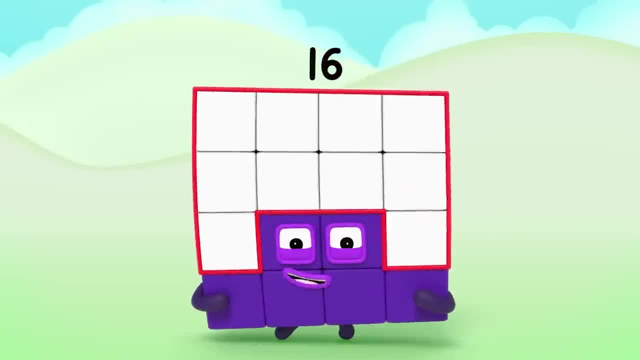 Wait, let me guess Square party one, two, three, four, five, six, seven, eight, nine, 10,, 11,, 12,, 13,, 14,, 15,, 16.. I am 16.. Square is a box And guess what? I've got 16 blocks. 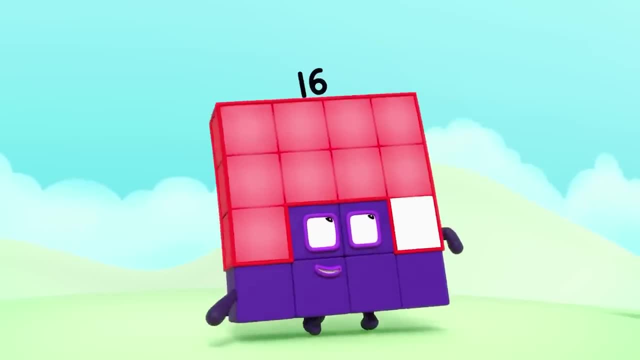 And that's how we make 16 squares. A square set will give one of us a without a button and two will give others a promptly Out of the boxocal只. seeing your wife, What happened that you're boish to doing with your son?